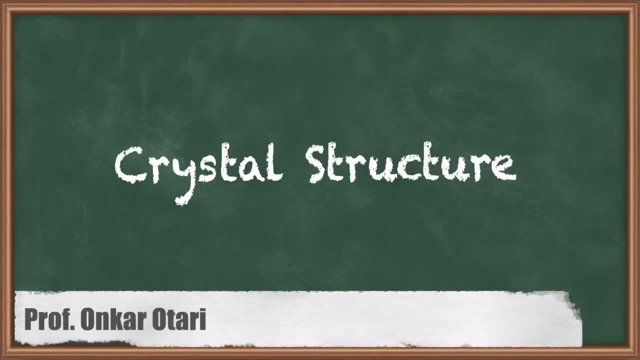 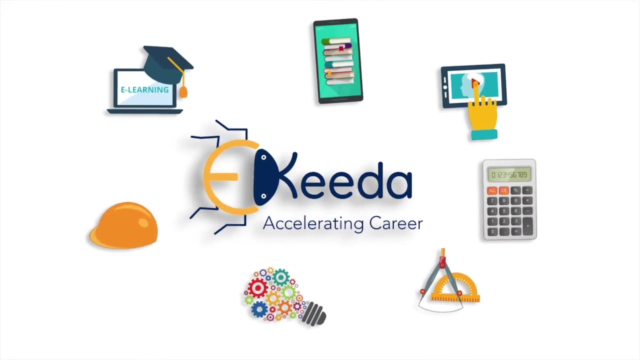 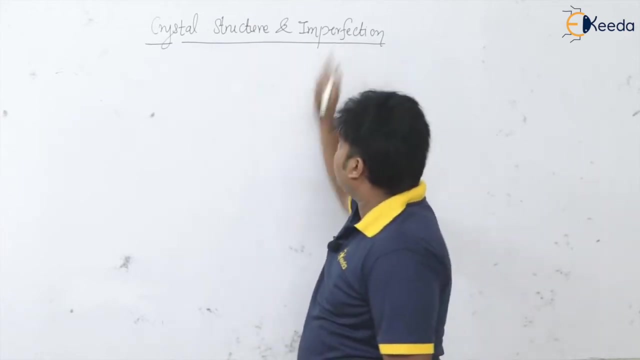 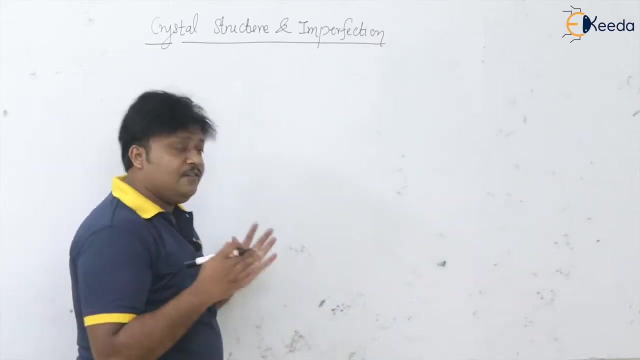 welcome students. now in this video we are going to start with our first topic of the subject, material science, that is, the crystal structure and imperfections. so definitely the first. we will talk about the crystal structure, then we'll talk about the imperfections in the crystal. so in this subject, material science, of course this is quite theoretical. 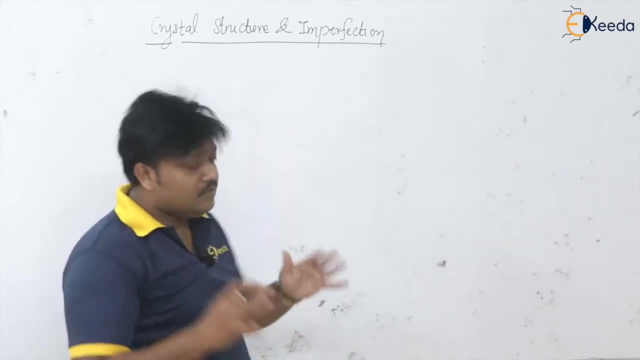 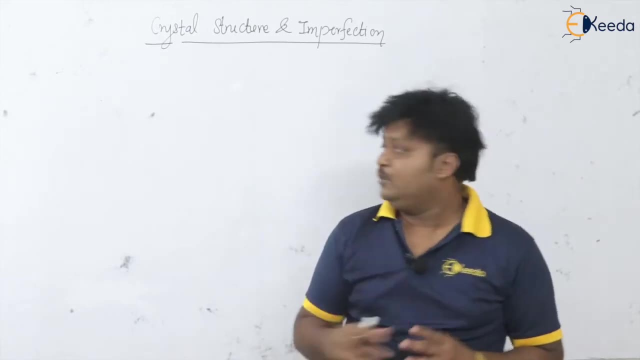 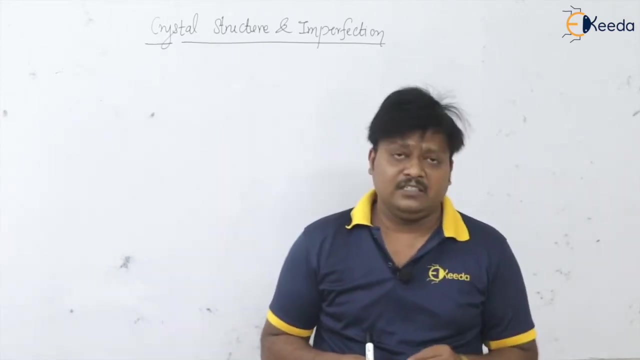 subject. so so whatever the uh, some short notes i will write to put uh onto the board. definitely so can. you can have, you can pause the video and you can see the important notes. okay, so see here. so crystal structure is what actually what it gives us. so it gives us. 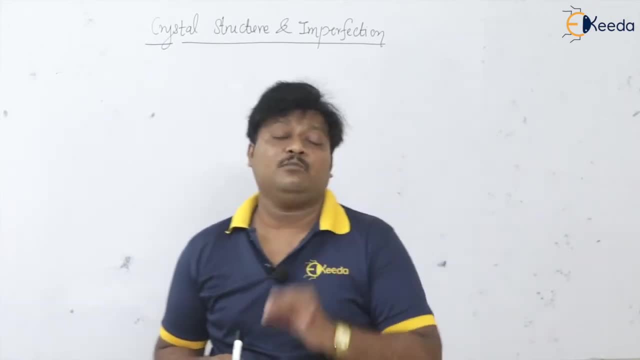 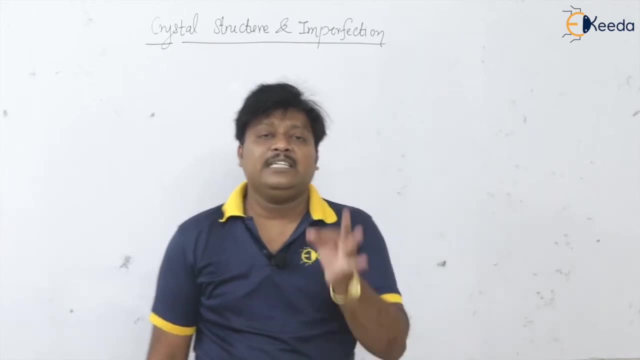 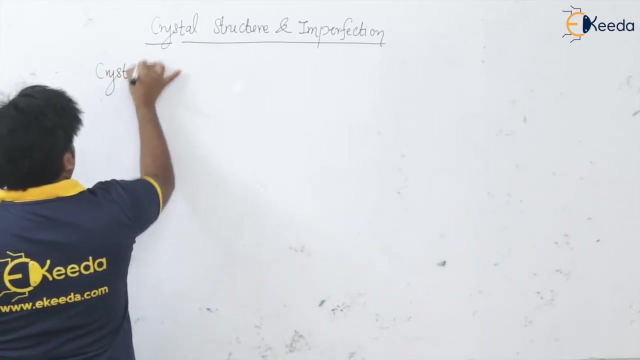 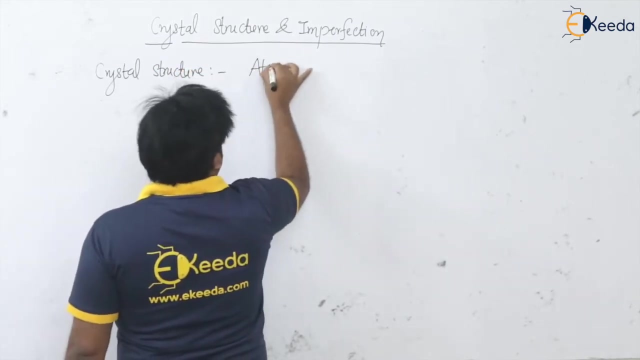 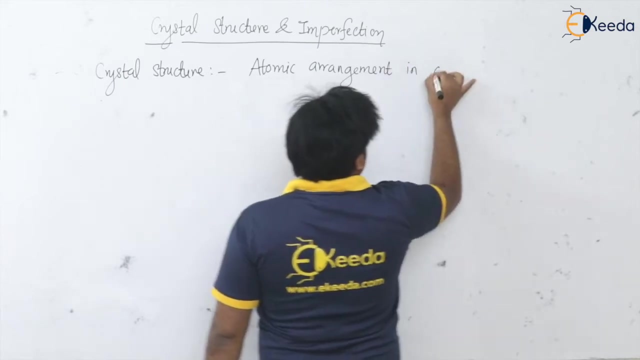 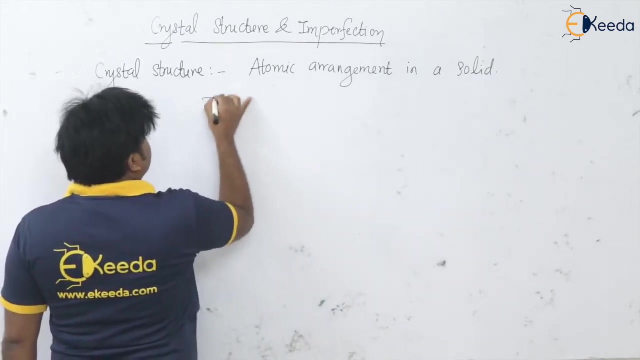 the atomic arrangements or the positions of the atom in a given solid body. okay, so crystal structure is nothing but the atomic arrangements of a solid. what is the crystal structure? we start with the crystal structure. so it is what it is: the atomic arrangement. atomic arrangement in in a solid, in a solid. what is this actually? so this is, this is. 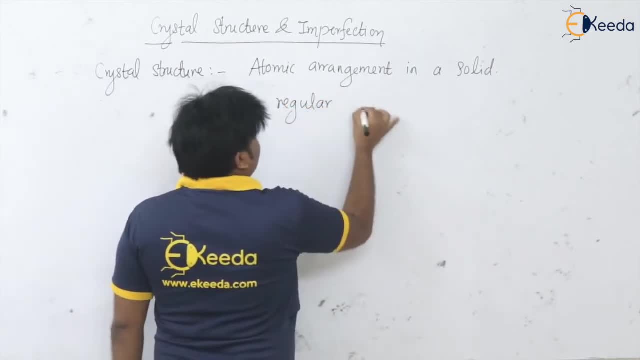 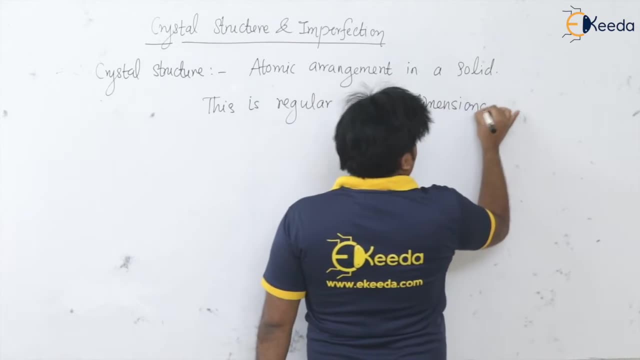 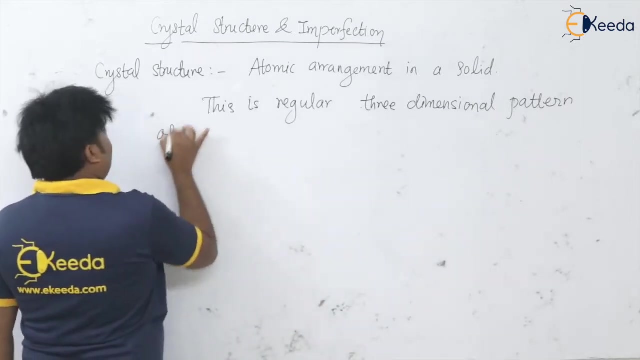 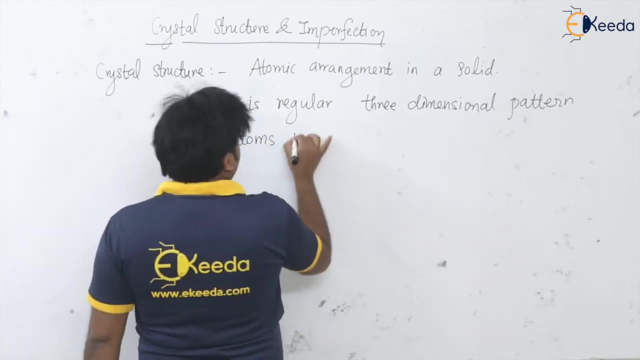 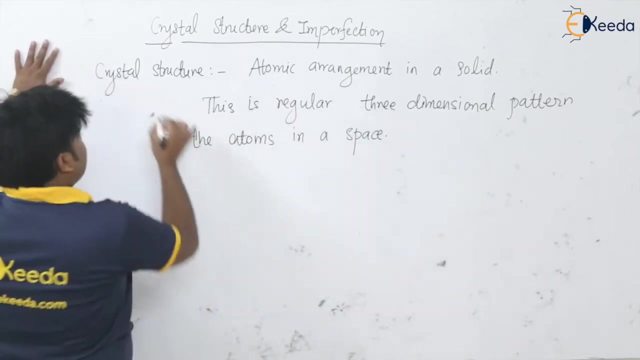 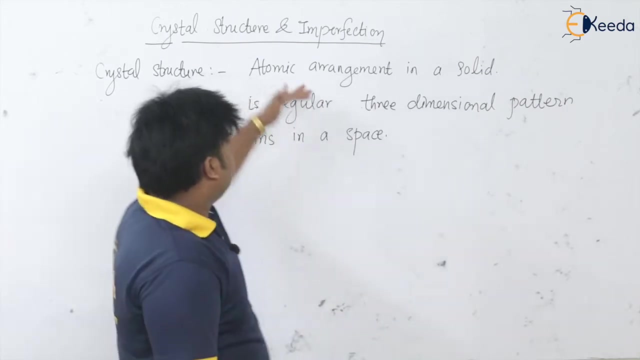 regular three-dimensional- this is regular three-dimensional patterns, 3d patterns of the atoms in a space. okay, so this is what the regular three-dimensional pattern of the atoms in a space- this is also the crystal structure- is going to give us. okay, with respect to space. 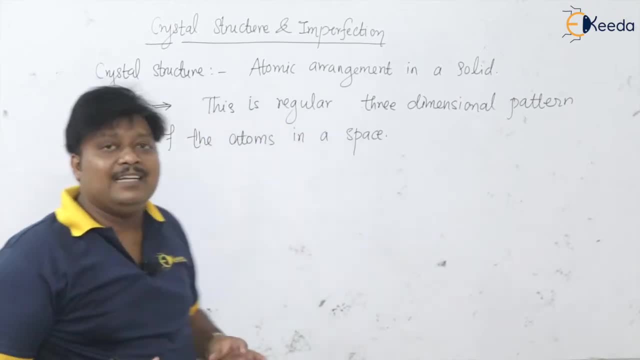 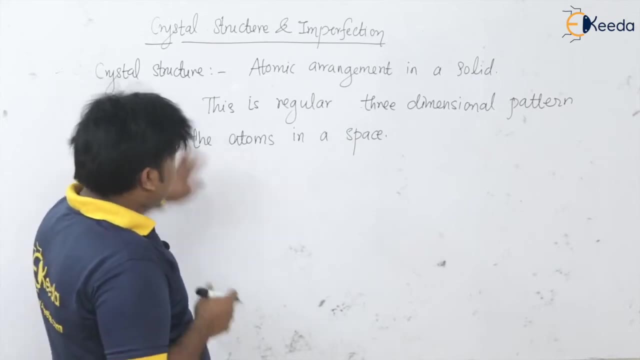 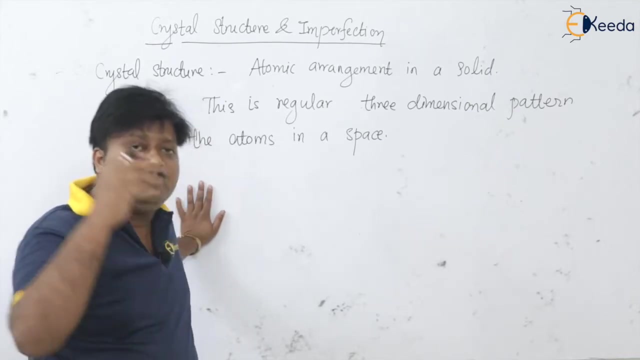 on the, say, a coordinates xyz axis. what are the how the atoms are arranged in this three-dimensional pattern? we can able to see, okay, by using this crystal structure now, why this regularity is going to come, yes, up to as a regularly given rma certain position. 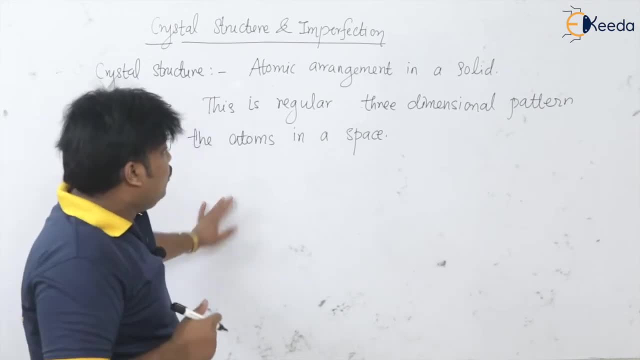 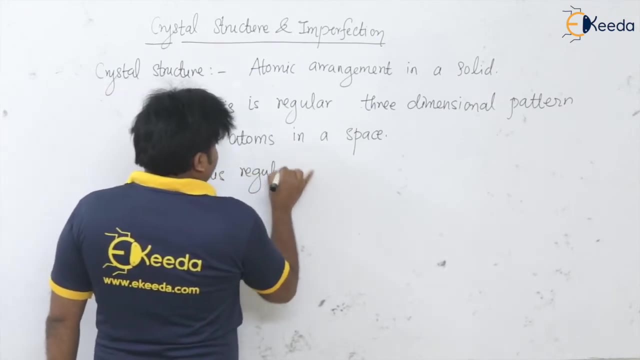 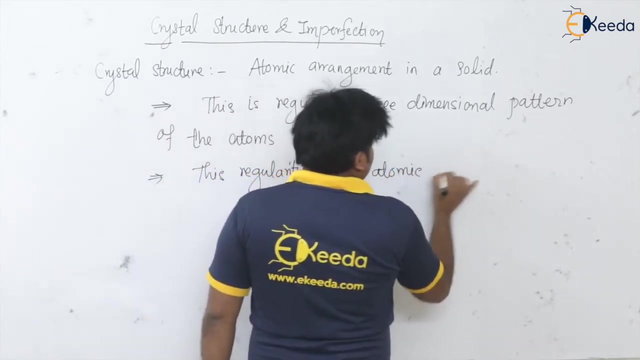 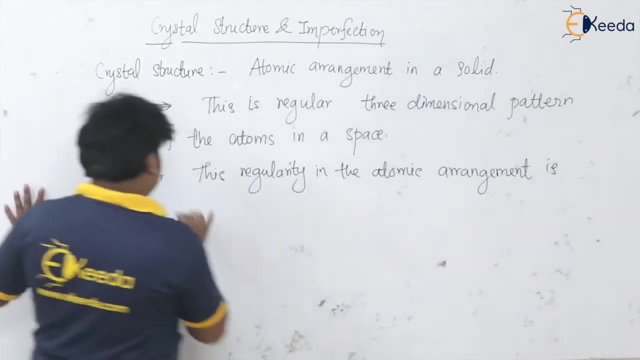 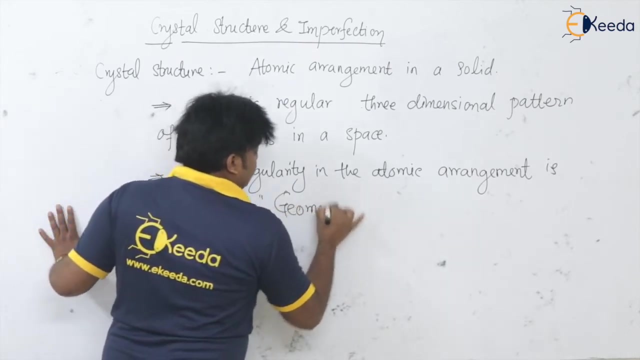 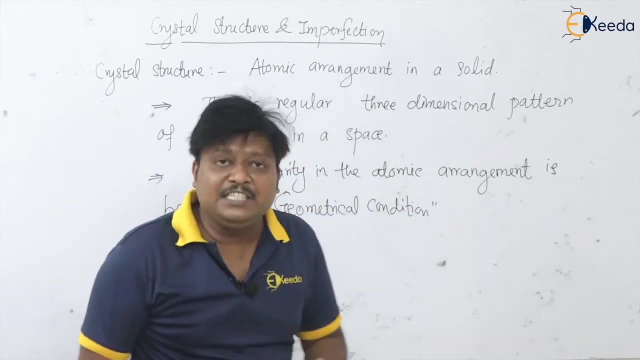 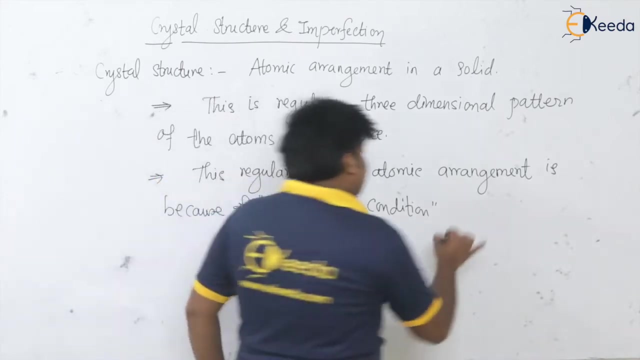 in the crystal structure. so see here, because this regularity, this regularity in the atomic arrangement, atomic arrangement is because of why, because of why the geometrical, geometrical conditions, why they are regularly arranged, because of the sub geometrical conditions and why these geometrical conditions which are imposed, which are 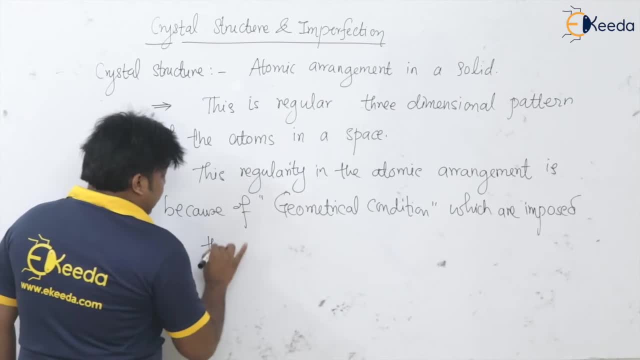 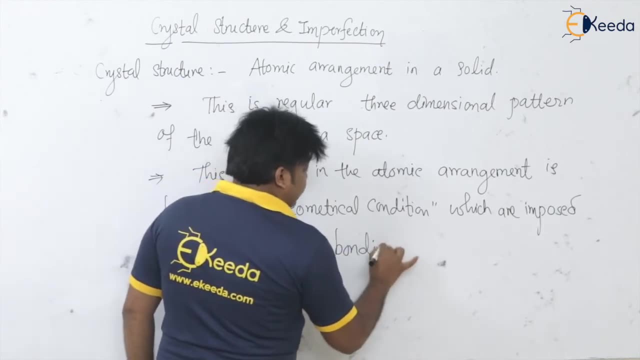 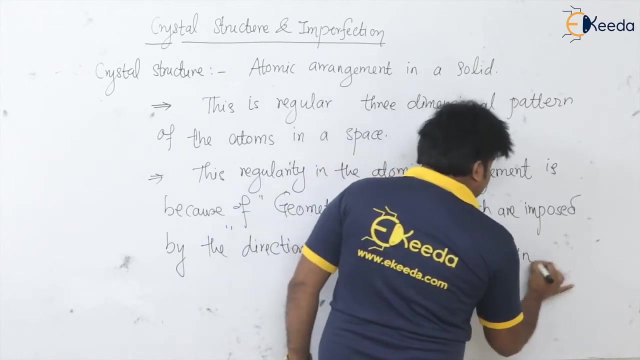 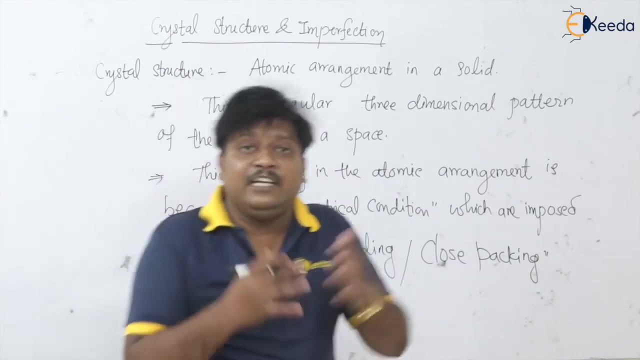 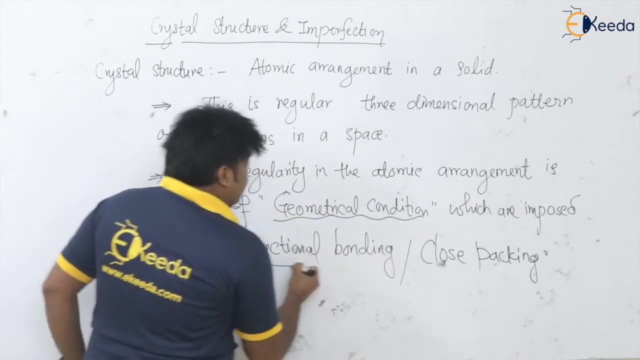 imposed by the directional, very important directional bonding. directional bonding or the close packing of atoms. the close, see, this is the reason why they are are orderly arranged, they are having the regularity in their arrangement, atomic arrangement- because of see the geometrical conditions which are imposed by some directional bonding and of 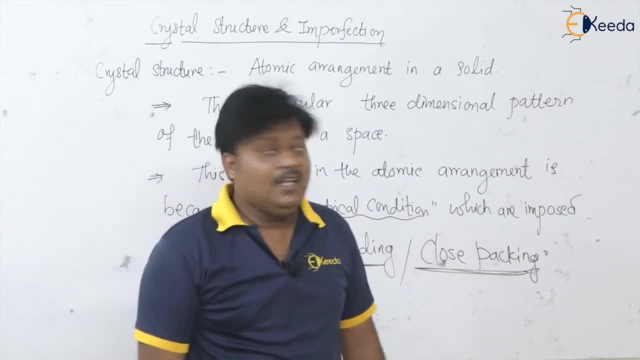 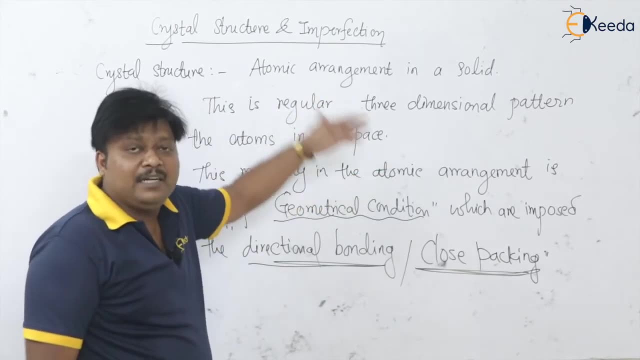 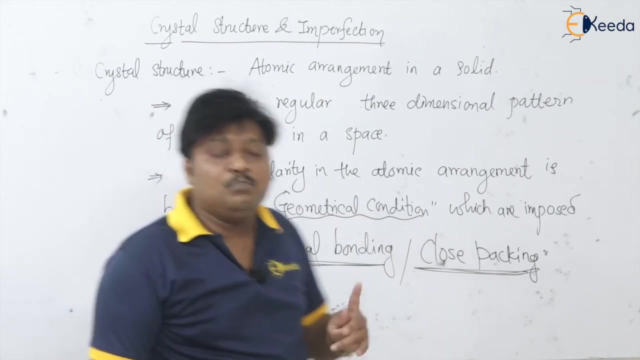 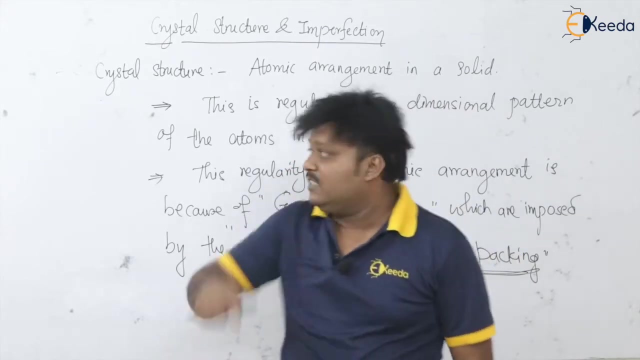 course they are closely packed. that is the main reason. this is the crystal structure, so atomic arrangement in the solid. we are getting the three dimensional patterns of the atoms in the space. and why they are regular? because the geometrical conditions imposed by the directional bonding or the close packing between the items. that is why we are getting this crystal structure. 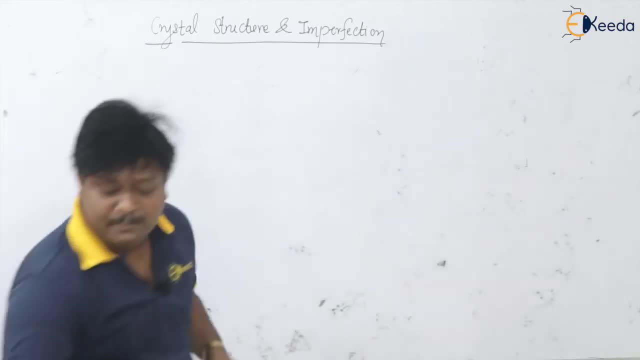 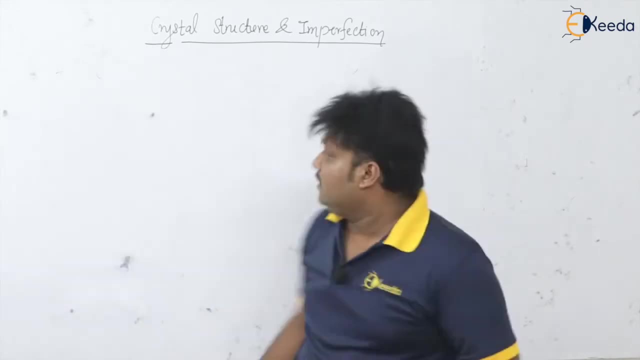 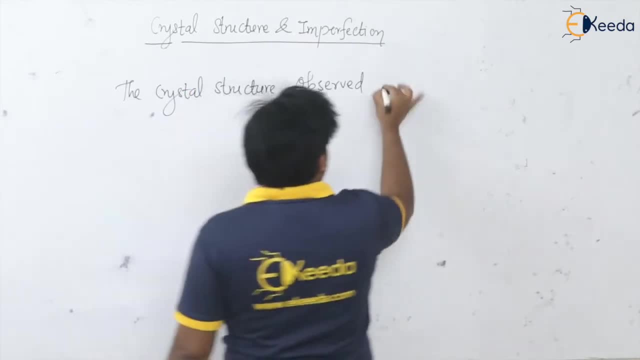 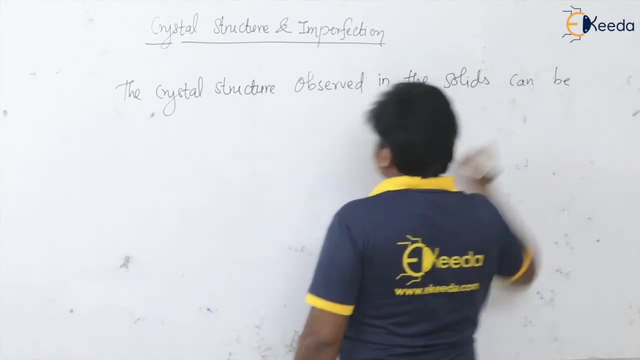 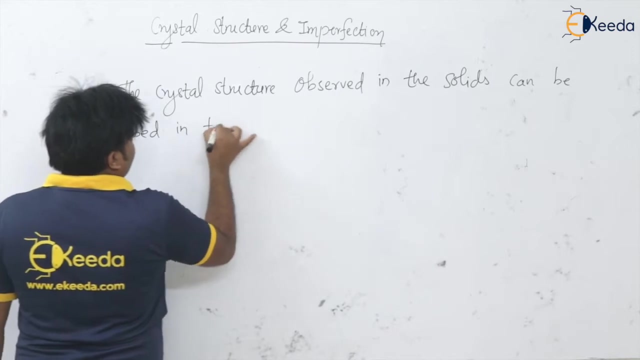 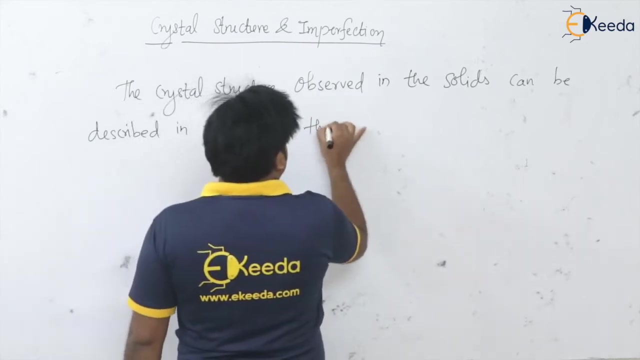 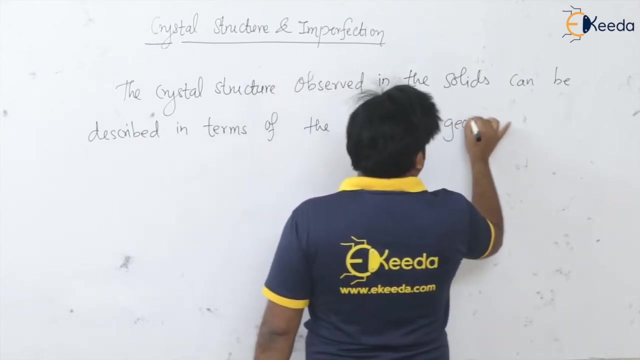 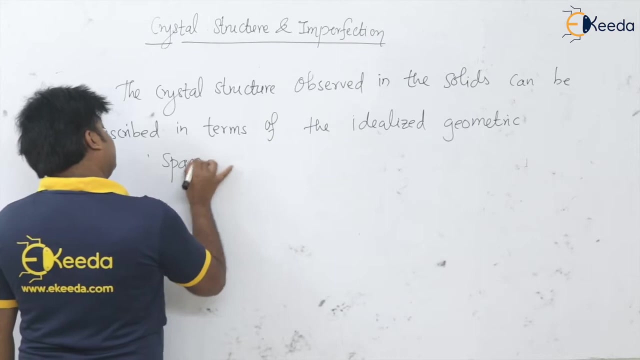 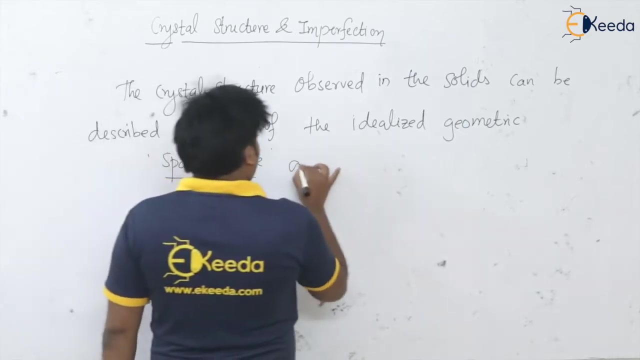 the, the, the crystal structure. so the crystal structures observed in the solid, in the solids, can be described. can be described in terms of. can be described in terms of the idealized idea. lies geometric, geometric space, lattice, space like this. see very important or. this space lattice is also known as, or the space that is also known as the point. 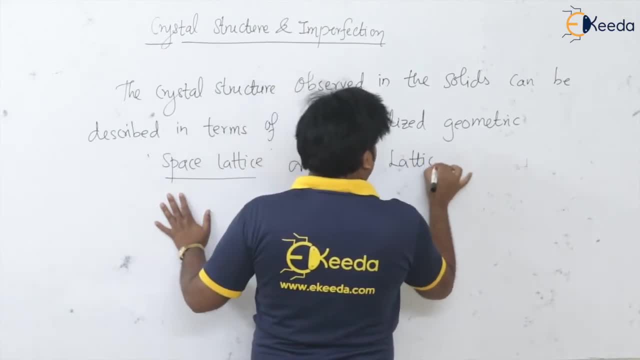 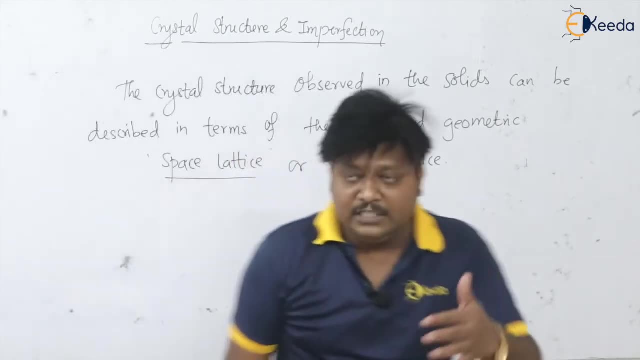 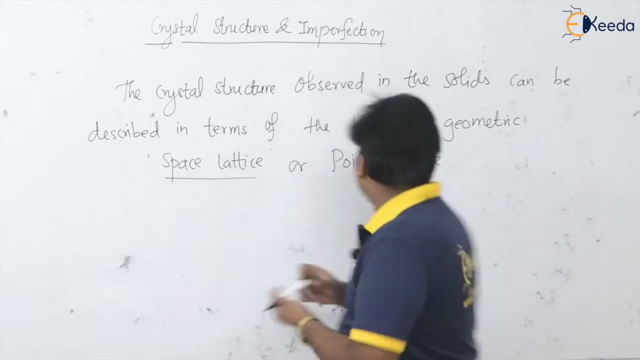 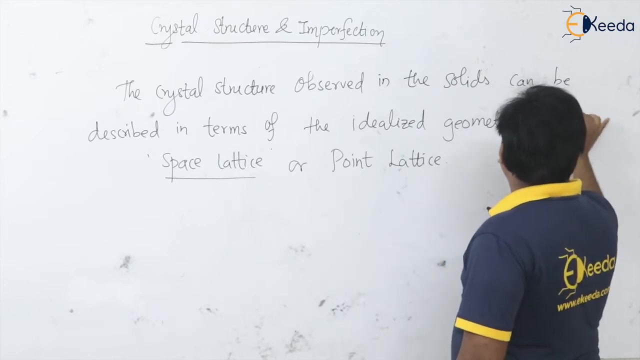 lattice, the point lattice or lattice, okay, so see here. so the crystal structure which are observed in the solids can be described, can be described in terms of the some idealized geometric condition. actually the idealized geometric condition, which is the space lattice, which is the space lattice, or 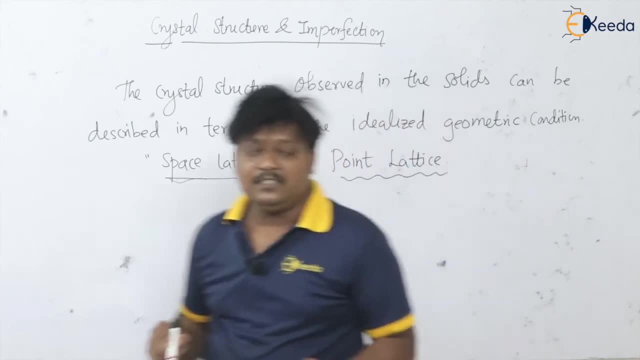 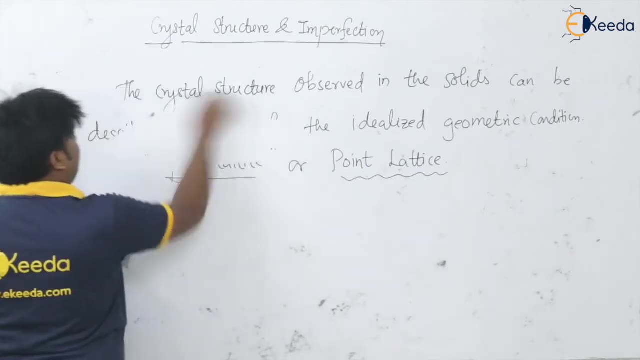 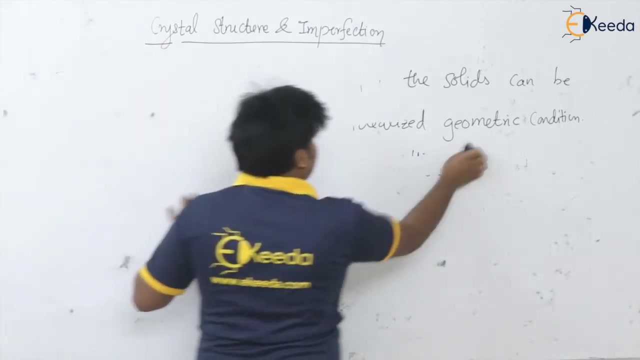 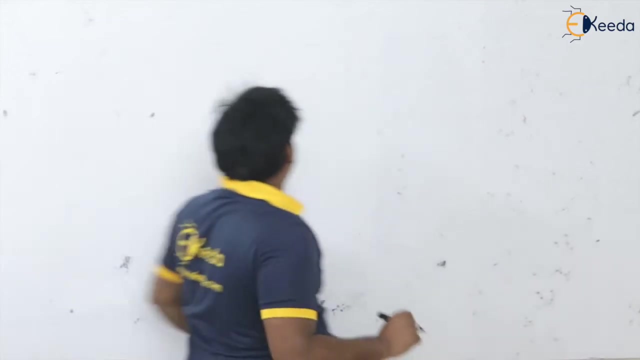 this is also known as the point lattice. so of course we can see here the space lattice how it look like, or point lattice. so we can see here the three-dimensional few of these atoms are arranged. so see how this space lattice or point lot is this look like. so very simple: have a tube, because we 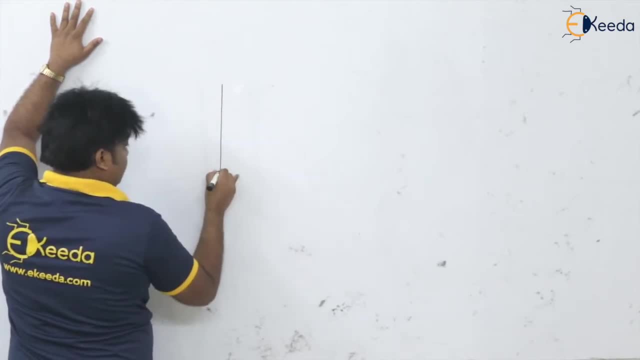 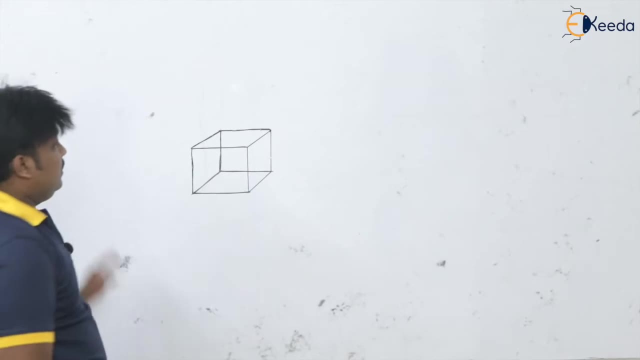 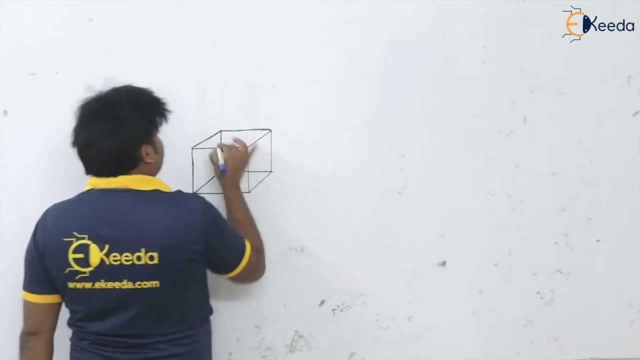 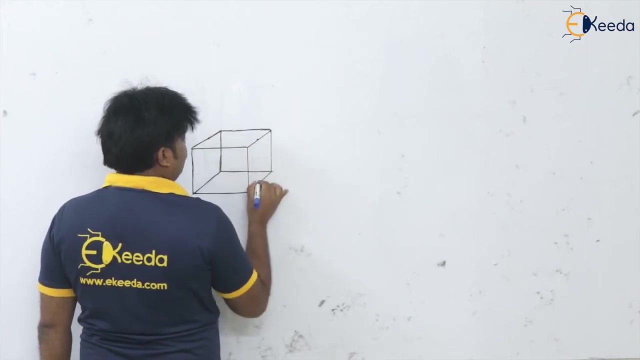 are going to see the three-dimensional pattern. I am going to draw here a cube, and so see your students. now I am going to show you here the point lattice or the space lattice here. so say, this is the cube. okay, I'll take the midpoints of. 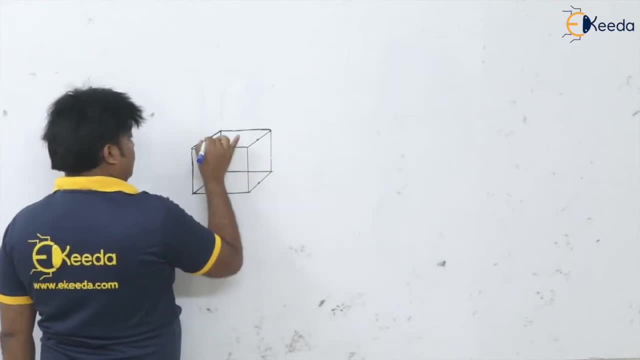 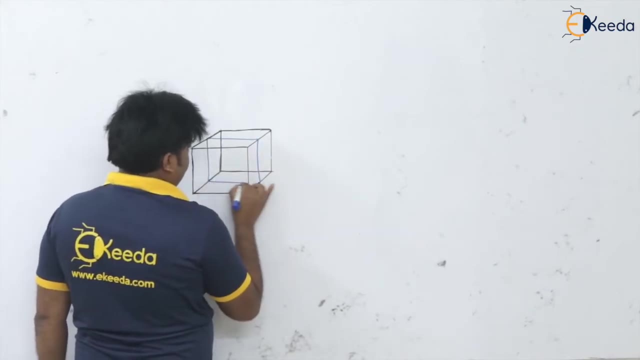 this. so I will create one more plane here at the center. then I will take, I will draw here, I will show you one more plane here at the center. okay, then I will take the center of each. okay, then I will take the center of each plane, plane. 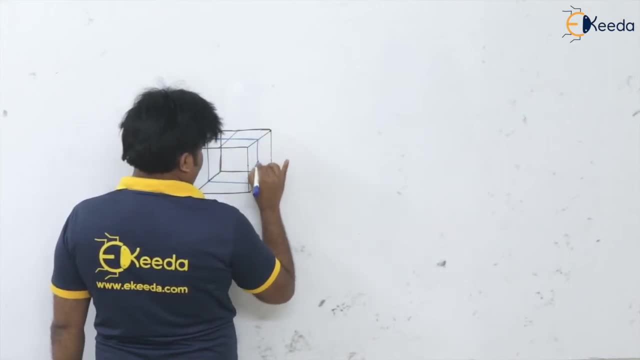 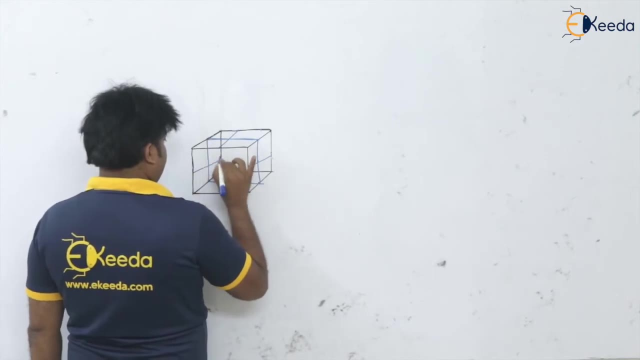 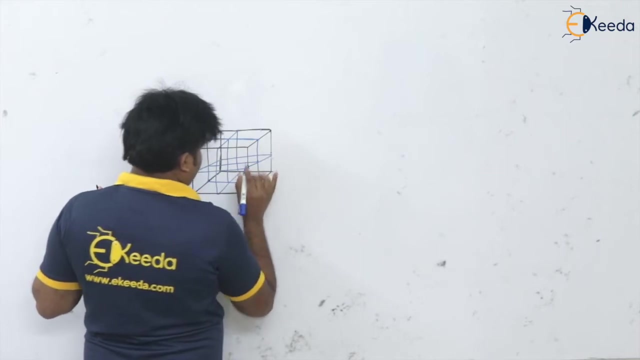 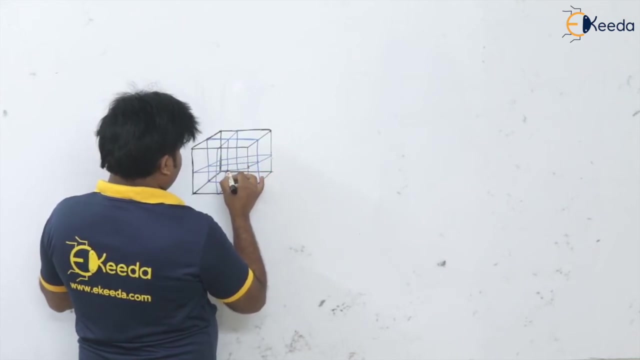 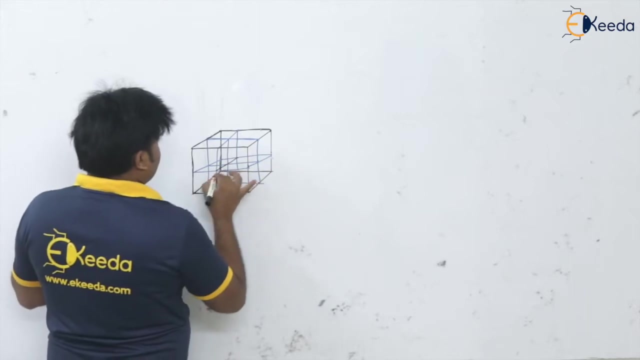 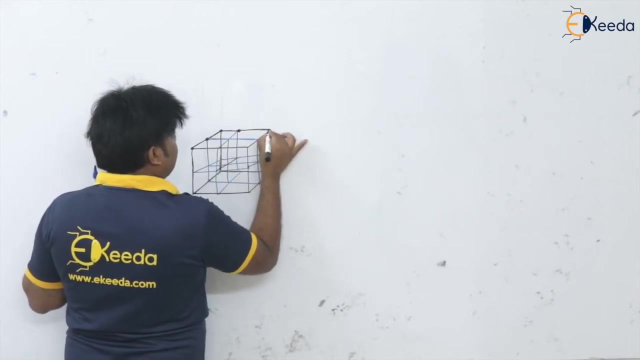 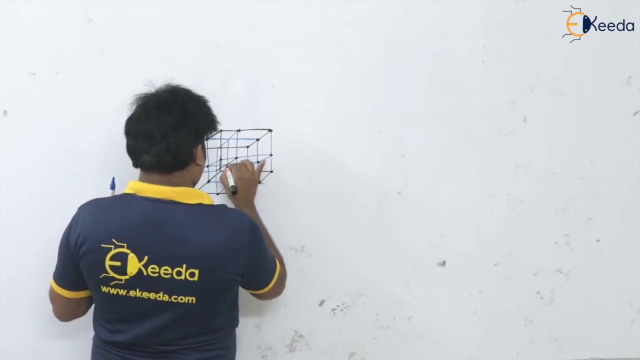 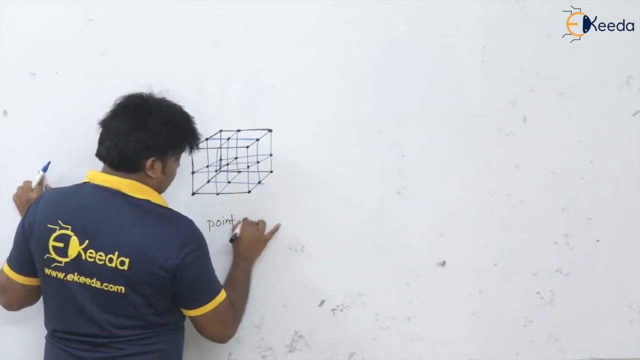 okay, then I will take the center of each plane. okay, now we'll join this. okay, and finally this: okay. so see, here we can get these, the atoms which are arranged in this space lattice. so this is the space or point lattice. this is the space or point lattice. 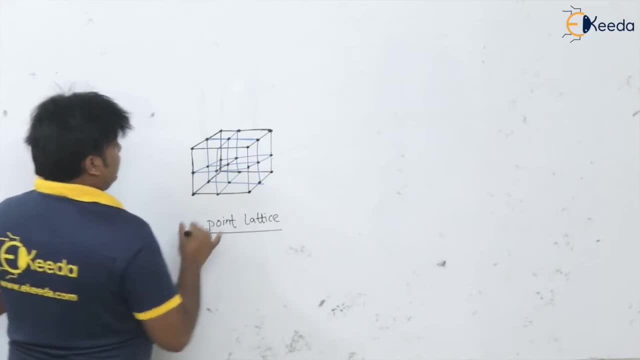 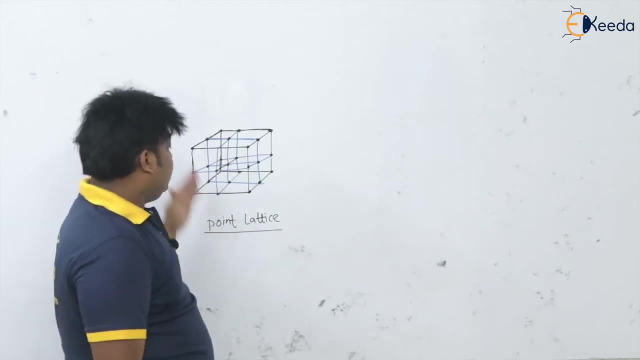 okay, so this is the space or point lattice. so this is the space or point lattice. 3d arrangement of the atoms. okay, and see. 3d arrangement of the atoms. okay, and see 3d arrangement of the atoms. okay, and see, here in this space lattice or in this: 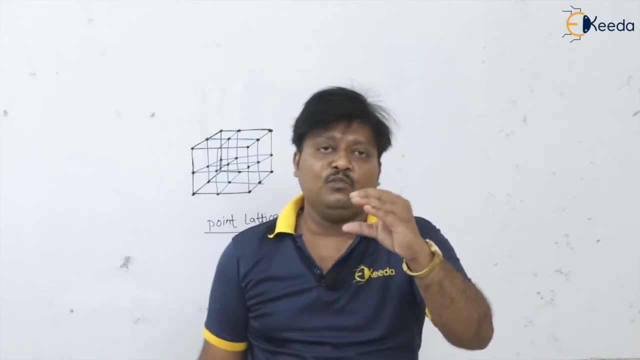 here in this space lattice, or in this, here in this space lattice, or in this point lattice, if we take the smallest point lattice, if we take the smallest point lattice, if we take the smallest volume of the space lattice, then that volume of the space lattice, then that. 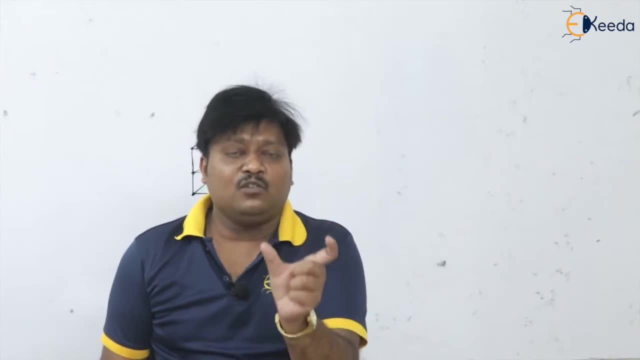 volume of the space lattice, then that smallest volume of the space that is is smallest volume of the space that is is smallest volume of the space that is is termed as or known as the unit cell, termed as or known as the unit cell, termed as or known as the unit cell. suppose in that, in this, suppose, if I 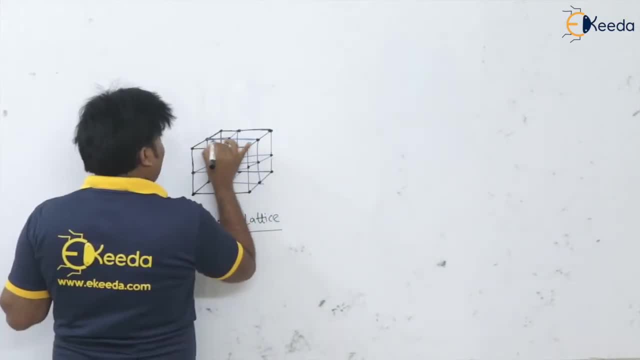 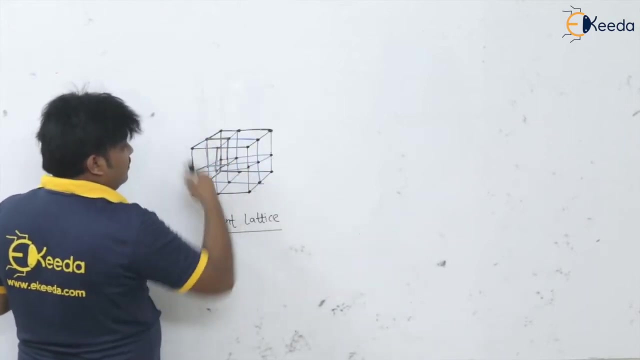 suppose in that, in this suppose, if I suppose in that, in this suppose, if I take this, I take this first small block of this here. I am taking this, okay, so for this point lattice which is big, okay, out of that I am taking this small, very small volume of this point lattice which. 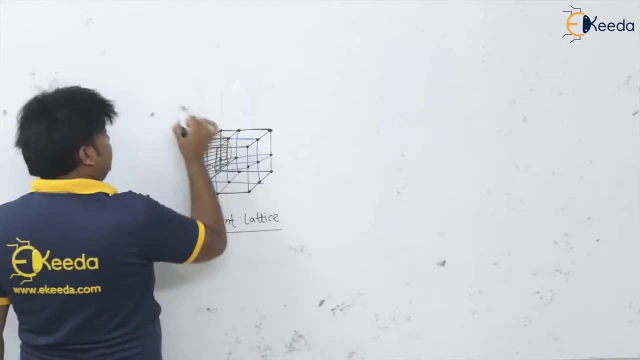 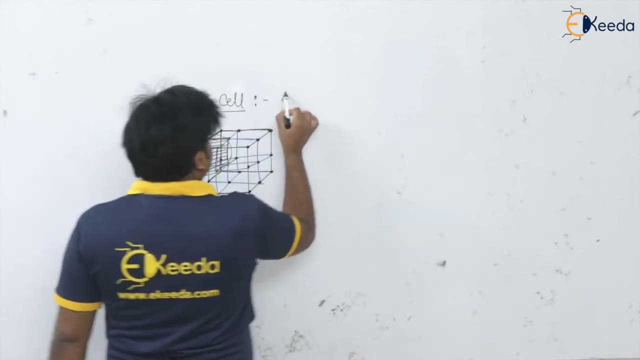 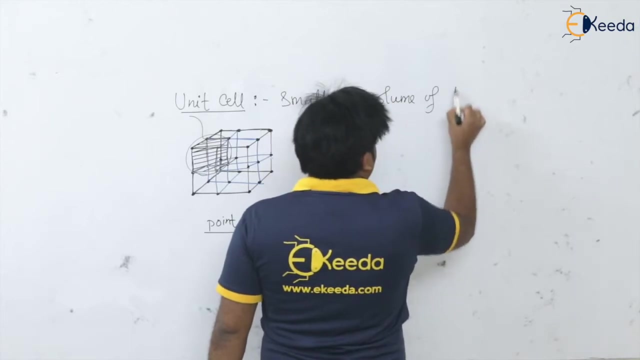 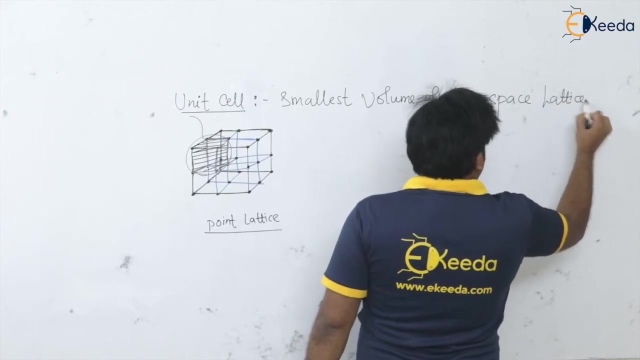 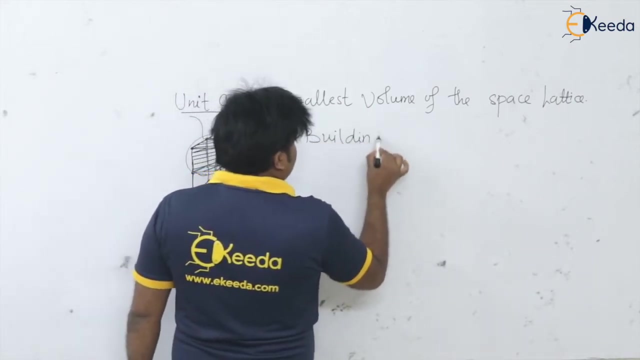 is known as, which is known as the unit cell, which is known as the unit cell. unit cell is what? the smallest volume of the smallest volume of the point or space lattice, space lattice, and which can be turned as capital scope? they are the building blocks. they are the building blocks if we arrange them, one or other, if we arrange. 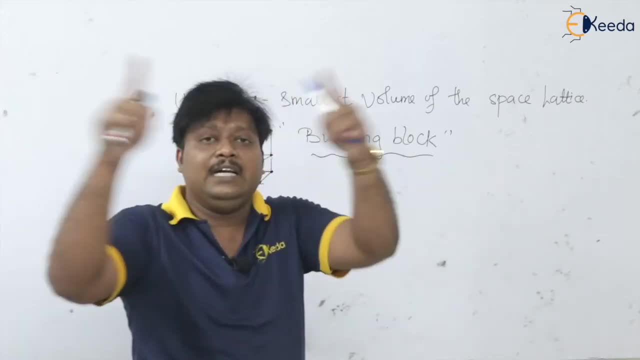 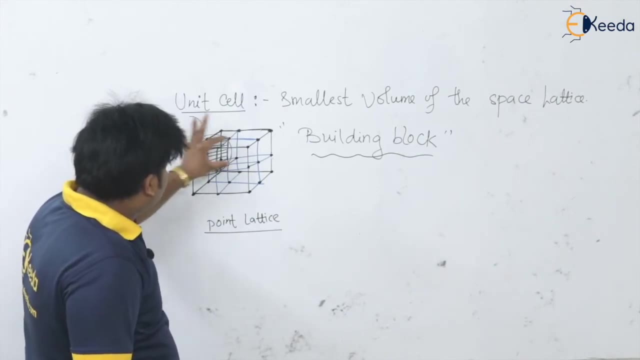 them one or other it these are going to form our point lattice here. so, but taking this as a smallest volume, if I keep this unit cell, one above the other and at the sides, then all together, all together, they are going to form, say, this is one unit cell behind that, one unit cell adjacent to this. 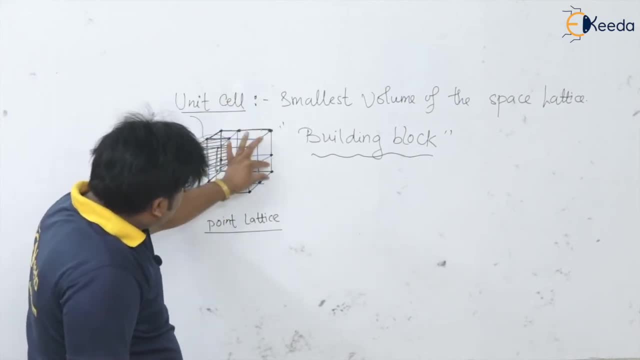 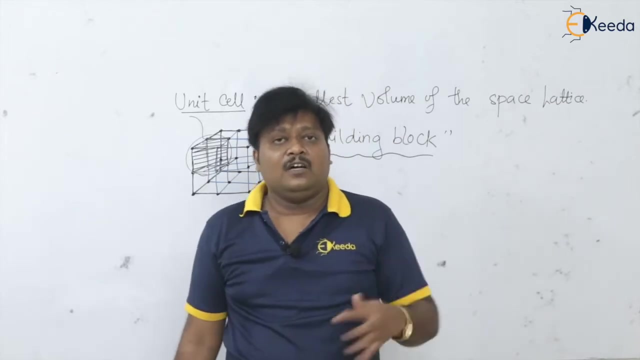 this is one unit cell. behind that, one unit cell, adjacent to this one unit cell, this is one unit cell. okay, so this is one unit cell. so, like that, by adding together all these unit cell, the space lattice is going to form. this is a very simple. we take the example of the building. so how this? the tall building. 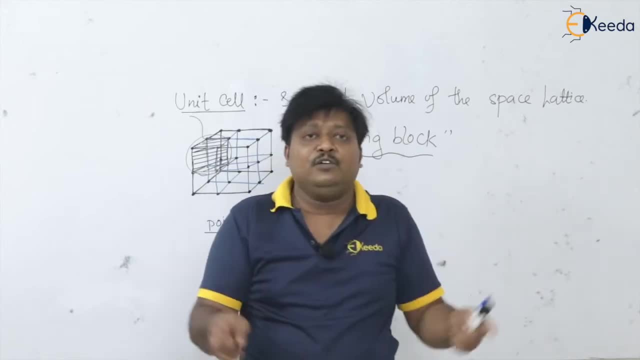 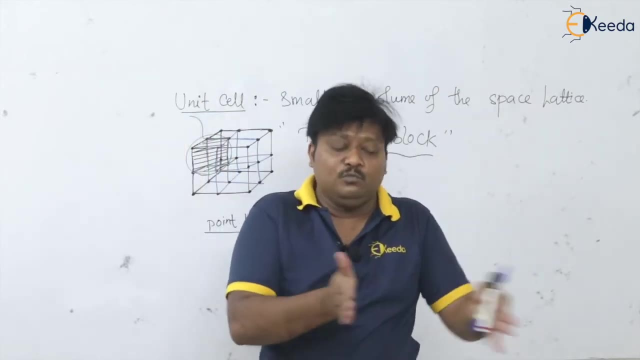 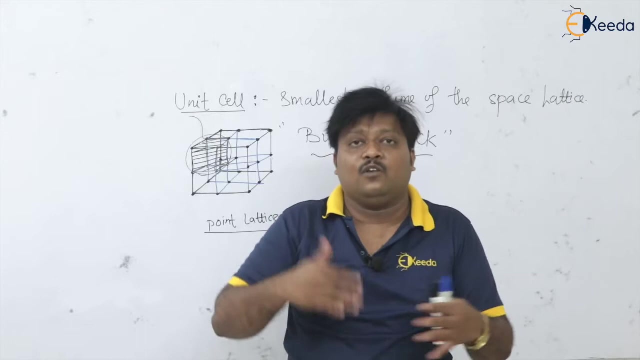 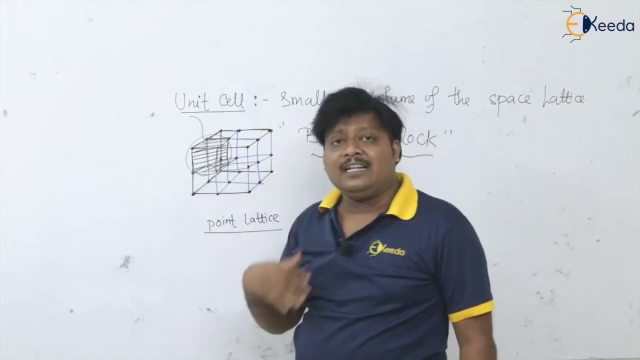 is going to form by. if every room in the building is its unit cell, that is smallest volume of this entire building. so these rooms in these building all together, one side side to each other or one above the other, like that, they are going to form the entire building. so the unit cells are also like that. 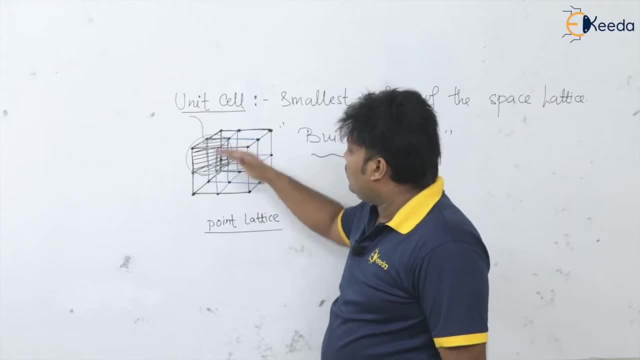 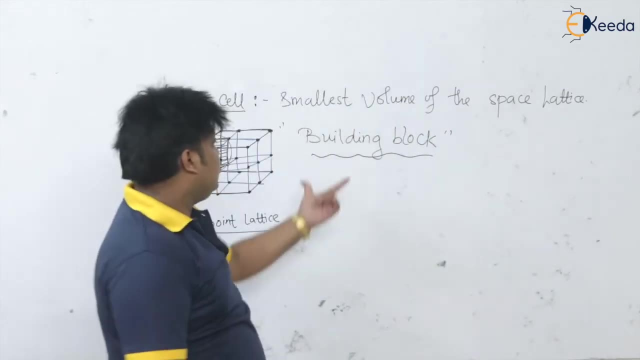 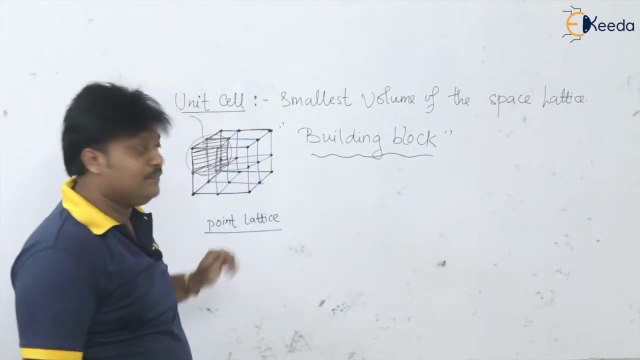 by arranging this unit, sell one or other adjacent to each other, the entire this space LaTige is going to form, so these are also known as the building blocks. okay, so this unit cell, this unit cell is going to look like. let us see this unit cell. i am going to draw here the unit cell. 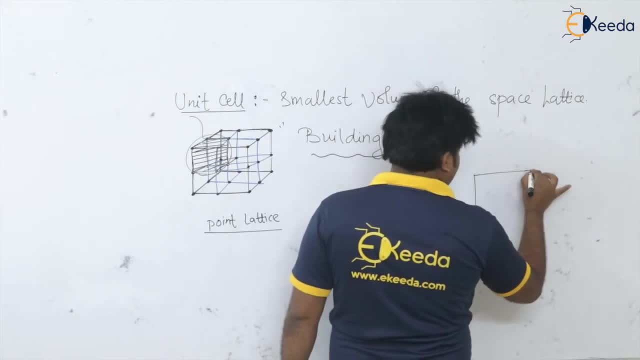 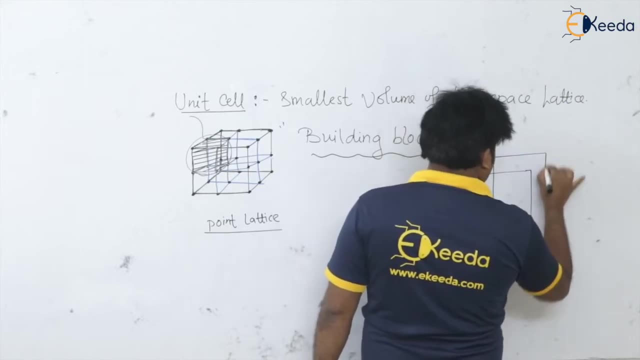 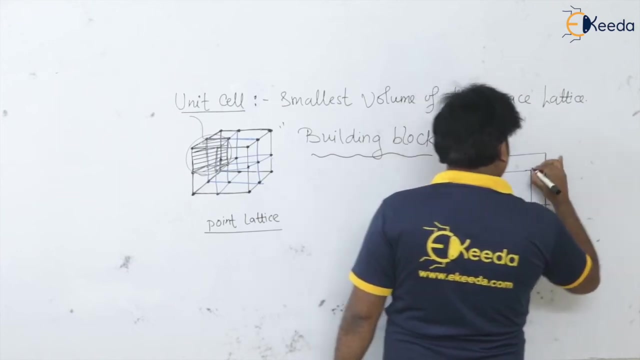 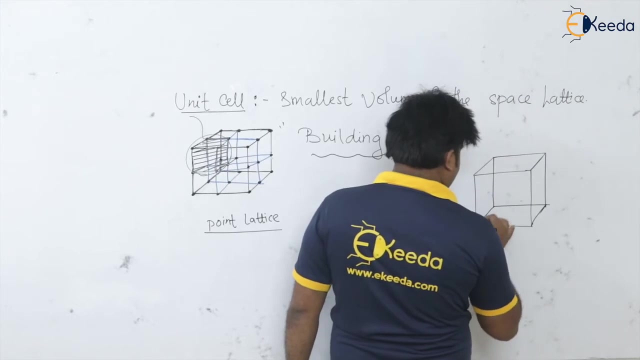 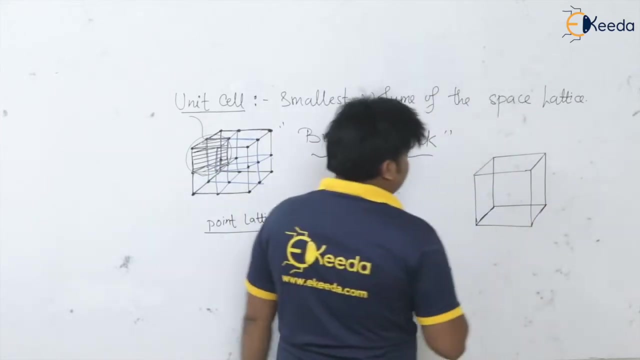 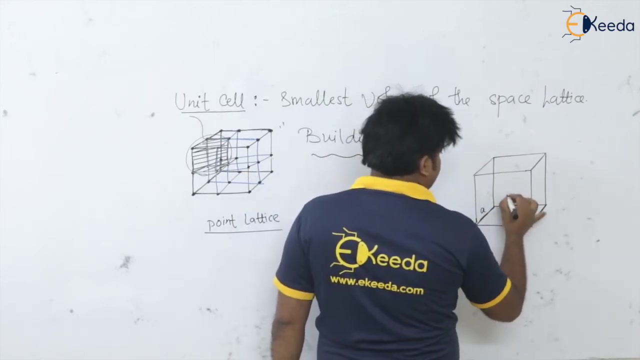 again, it is a cube. so see here: this is the one unit cell i am taking here. now see for this unit cell. we are having the crystallographic axis, say this is a, b and this is c, and the angle between these we can have this is alpha, this angle is beta and this 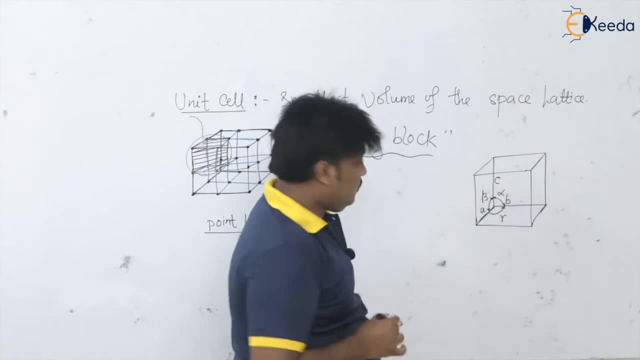 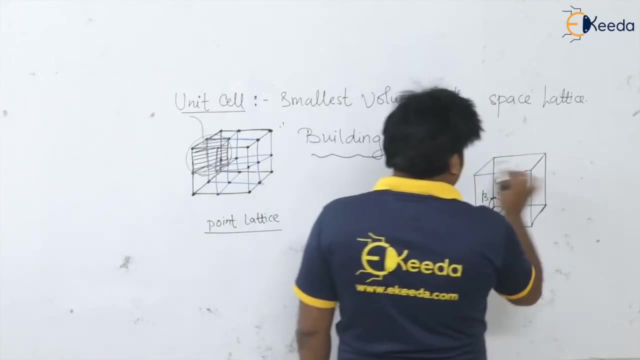 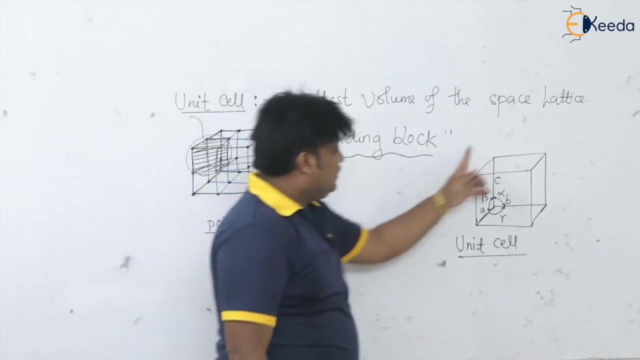 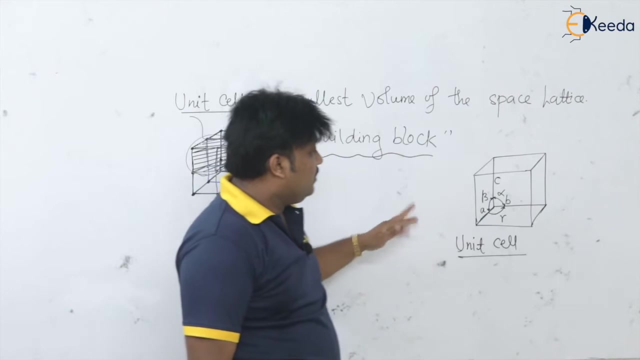 angle is gamma. okay, this is the unit cell. this is the unit cell. so a, b, c are the crystallographic axis, or we can have. these are the lattice parameters and the angle between this crystallographic axis. we are having alpha, beta and gamma. now see, based upon the relationship between this, a, b, c, 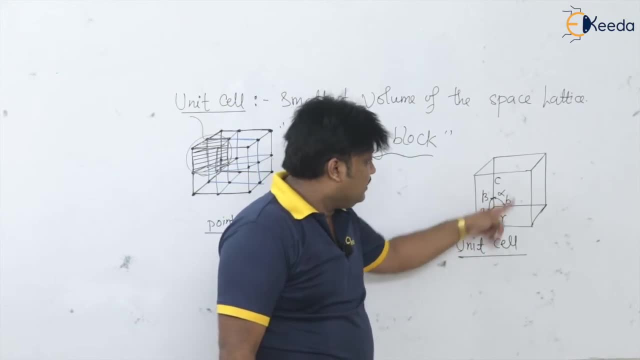 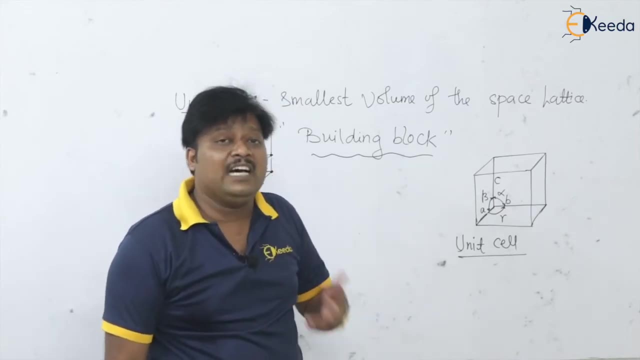 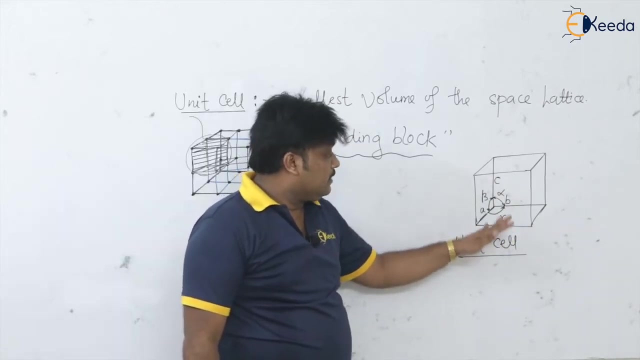 and the angle subtended by these three axes, we can have the 14 different arrangements or the arrays of this unit cell. so see, here, this unit cell is having this crystallographic axis a, b and c and the angle between this axis, okay, is alpha, beta and gamma, based upon the relationship between these crystallographic 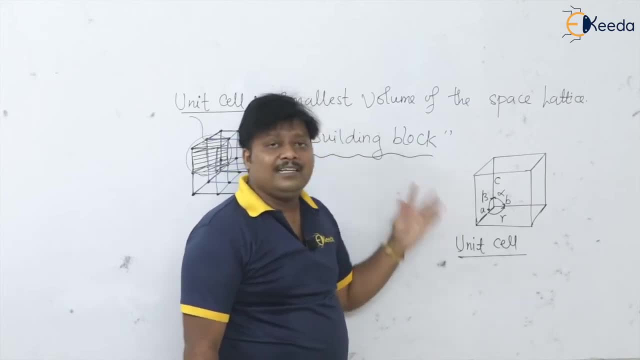 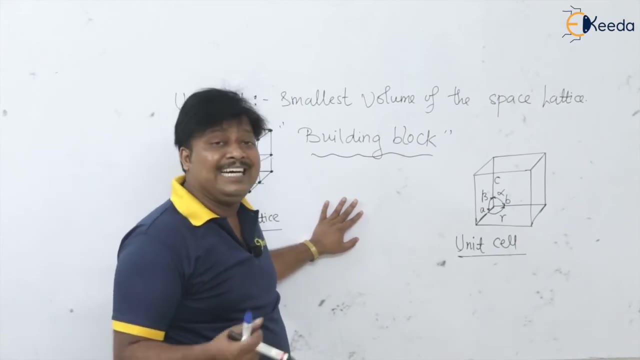 axis or the lattice parameters a, b, c and the angles alpha, beta and gamma. there are 14 arrangements or 14 arrays which are possible, was given by the french mathematician a, j, brevis, and these the brevis lattices. that definitely we are going to see what. so, based on this relationship between 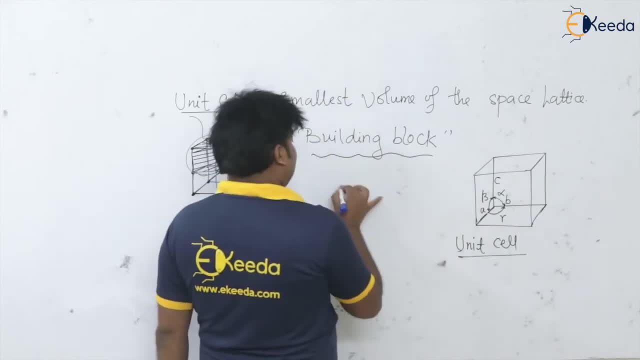 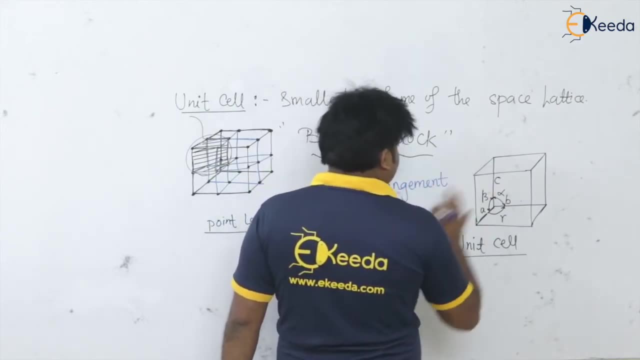 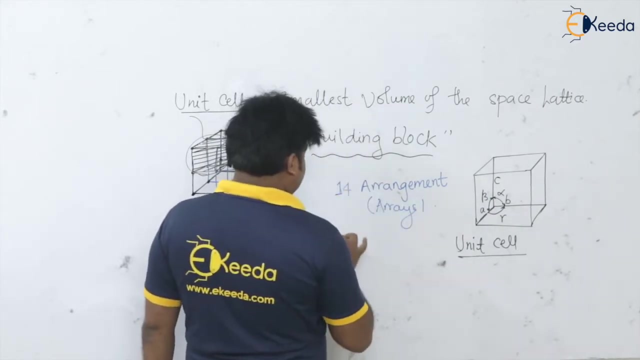 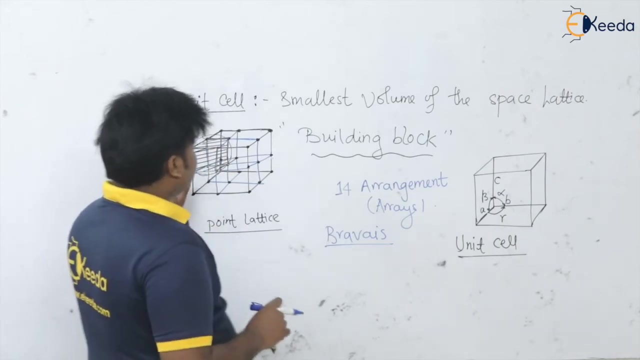 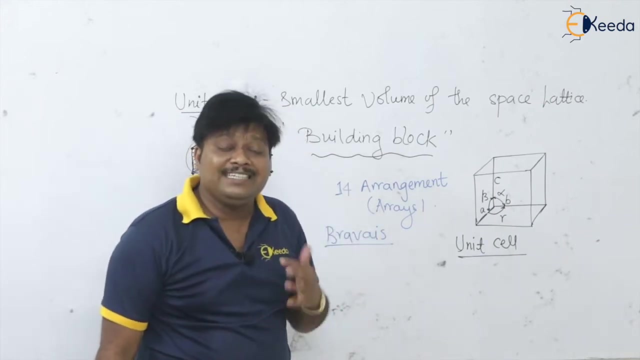 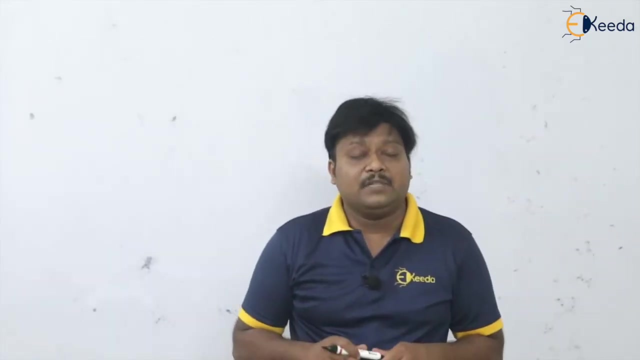 these axes and the angles. we are going to have 14 arrangements in the unit cell or arrays, which was given by brevis, a french mathematician, and, of course, these are the arrangements will be given for the seven crystal structures that we are going to have. dear students, now we are going to see these seven kind of crystal. structure and the 14 brevis arrays or arrangements in this, seven crystals and 14 brevis lattices. so let us take the first one, that is, the cubic structure. this is the cubic structure, that is the first one. so in cubic structure we are having this: a is equal to b is equal to c and the angle alpha is equal to beta. 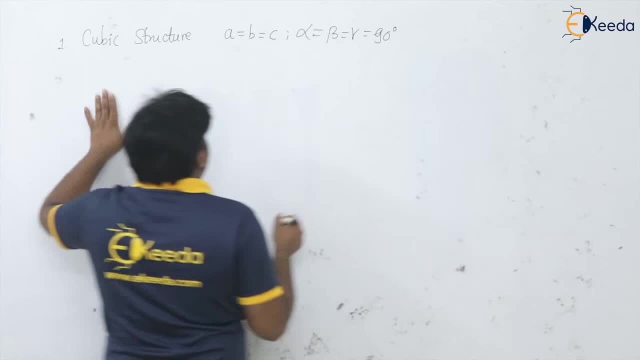 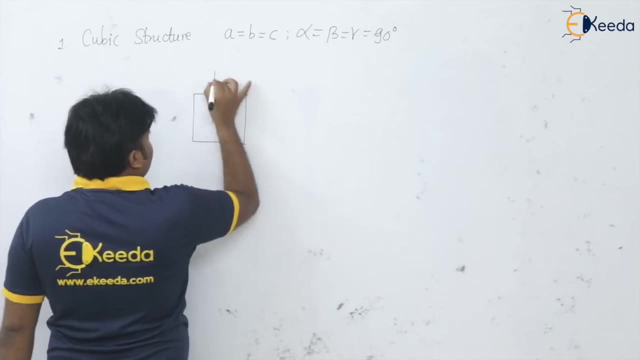 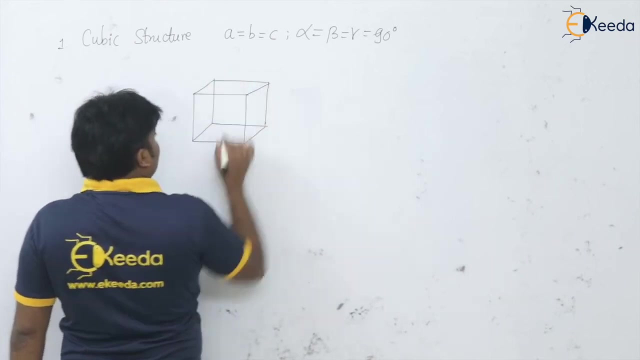 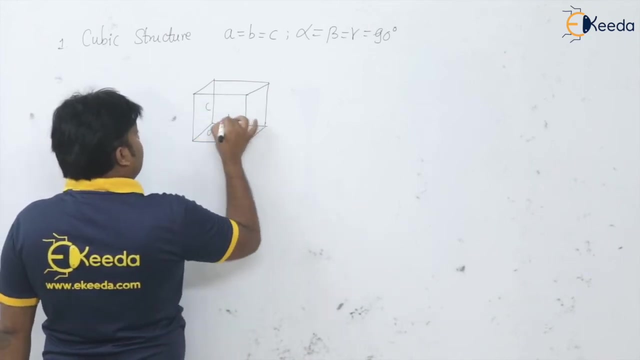 is equal to gamma, are 90 degrees, and see here. so this is a, a, this is b and this is c, these all are equal and this angle, alpha is equal to beta is equal to gamma is equal to 90 degrees. so this is a cubic structure in that we are having. what are the lattices? brevis lattices. 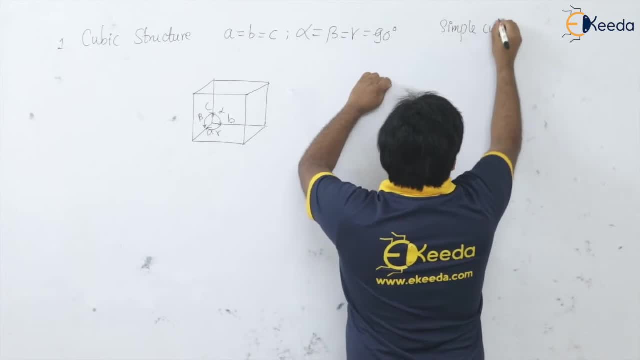 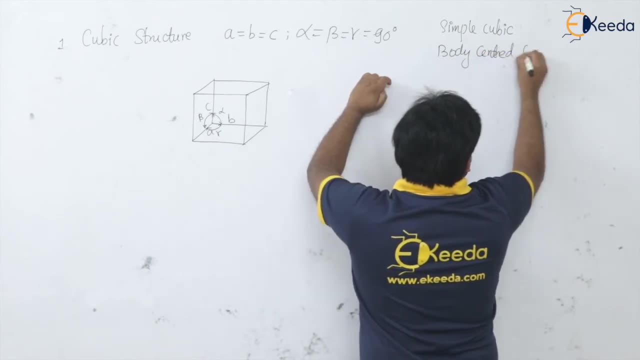 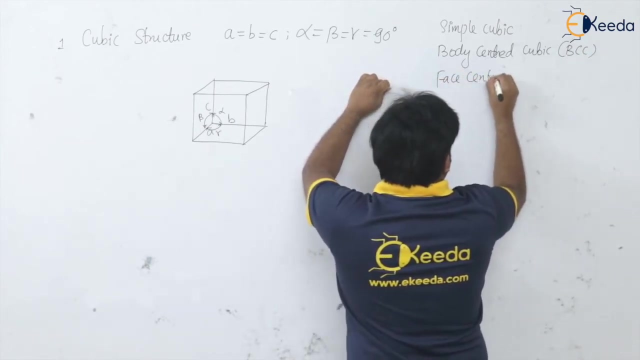 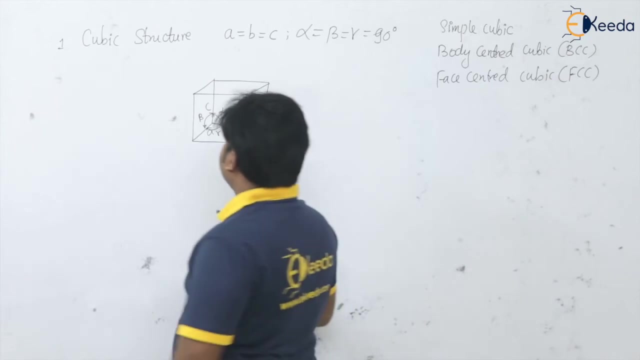 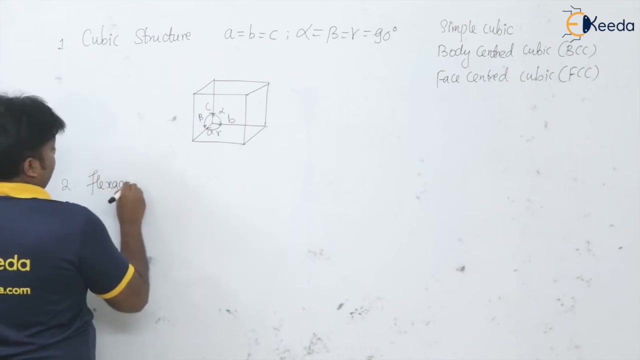 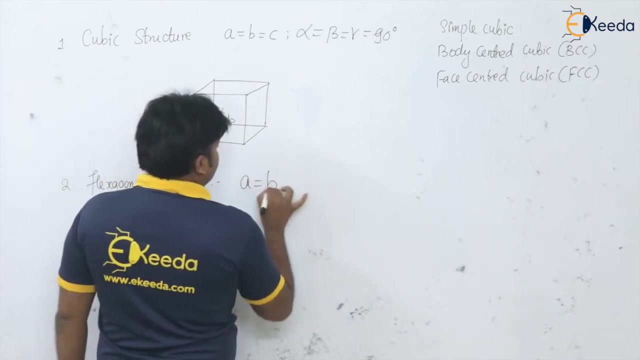 this simple cubic, simple cubic structure is there. then we are having body centered cubic, that is bcc. then we are having the face centered cubic, that is fcc. so this is the cubic structure. then we are having second structure is the hexagonal hexagonal structure where a is equal to b but not equal to c, alpha is equal to beta is 90 degrees. 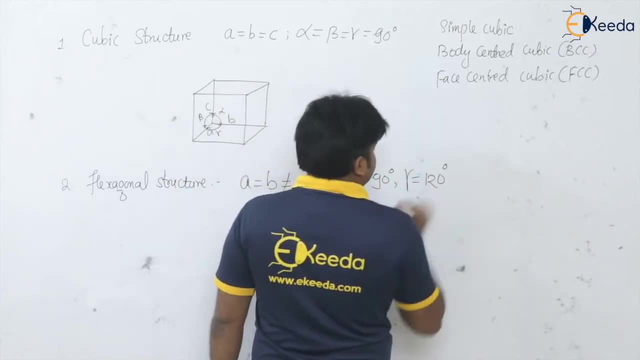 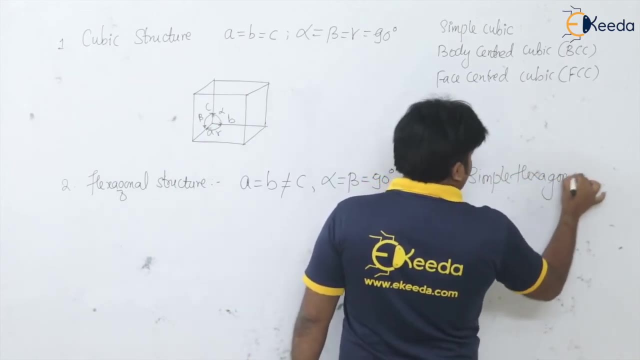 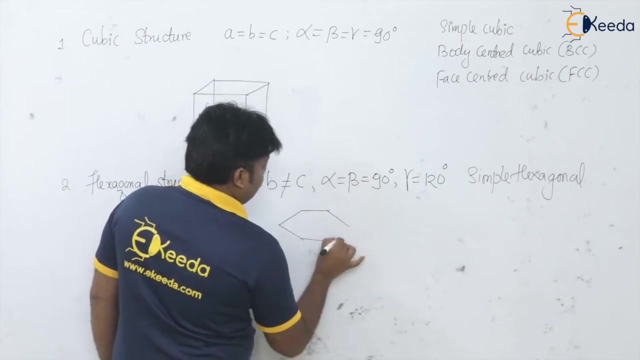 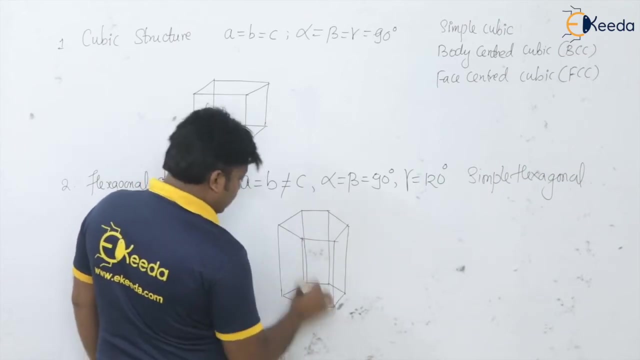 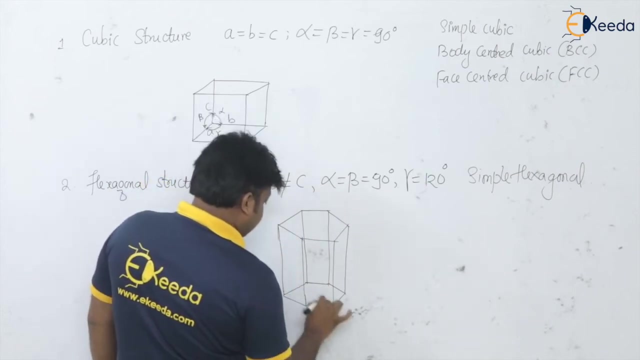 and gamma is 120 degree. and here we are having simple hexagonal structure, simple hexagonal. if you see the diagram, this is the hexagonal structure. okay, so this is say, this is a, this is b and this height- if i have this height- c, where a is equal to b, 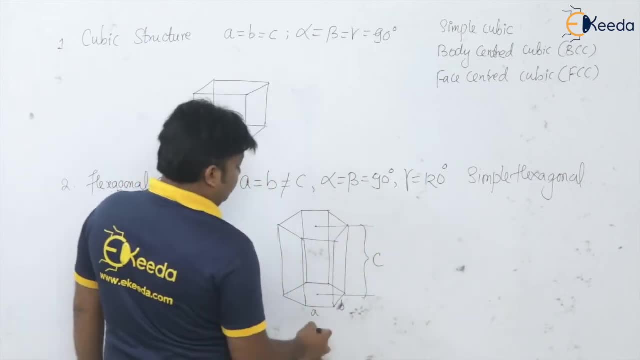 and this angle is 120 degree. so this is the hexagonal structure. so this is the hexagonal structure. this is the hexagonal structure. two on the f by the angle of angle of c. this is not the vector, but b is not equal to c. how I know to correct the equation? 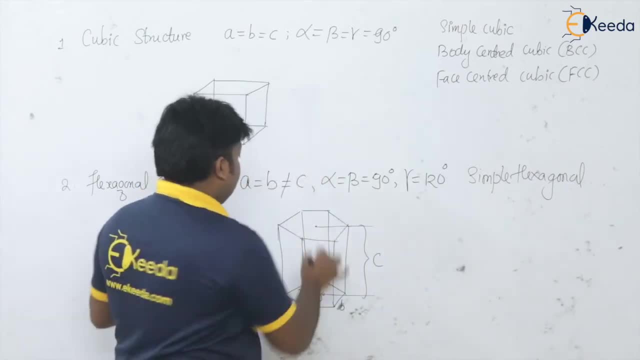 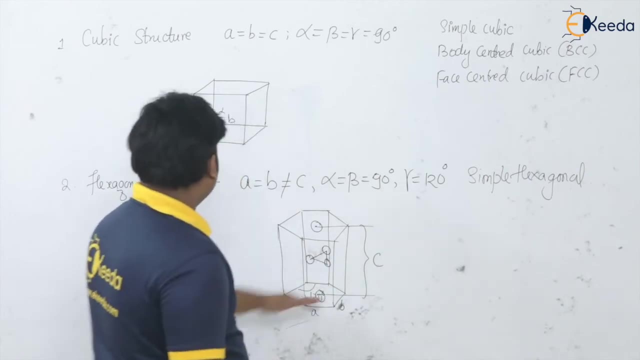 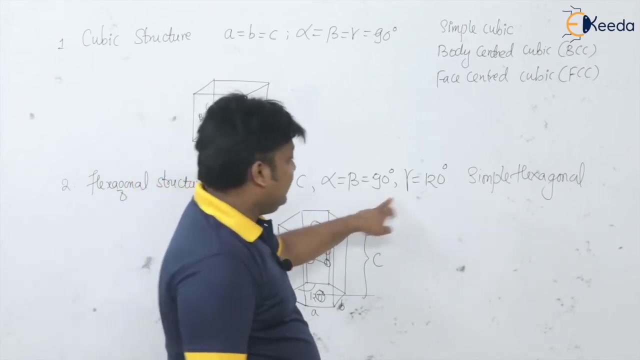 okay, so this is the hexagonal structure. twelve atoms at the corners, two on the face and three interior. this is the hexagonal structure. a is equal to b, but b is not equal to c. alpha, beta angles are 90 degree and gamma it is predetermined angle, which is 120 degree. 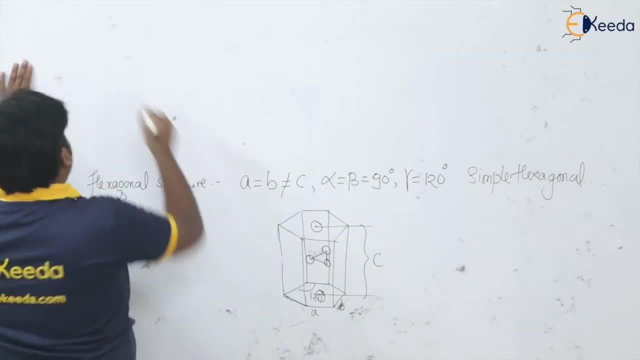 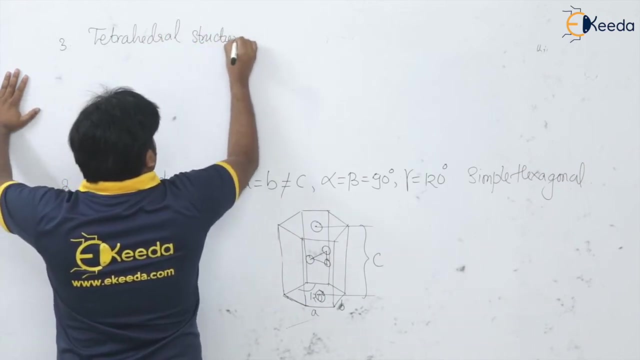 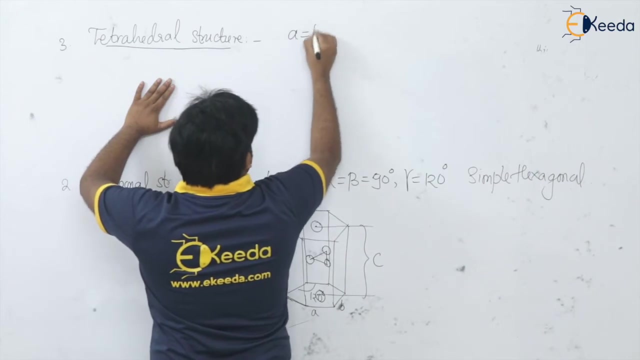 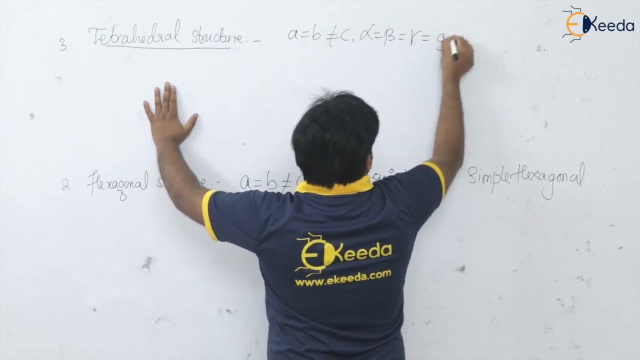 then the hexagonal. we will hexagonal, we will have the third, that is the tetrahedral. tetrahedral structure. So in tetrahedral structure, again same, this a is equal to b but not equal to c. but here all the angles, alpha is equal to beta is equal to gamma are 90 degrees. 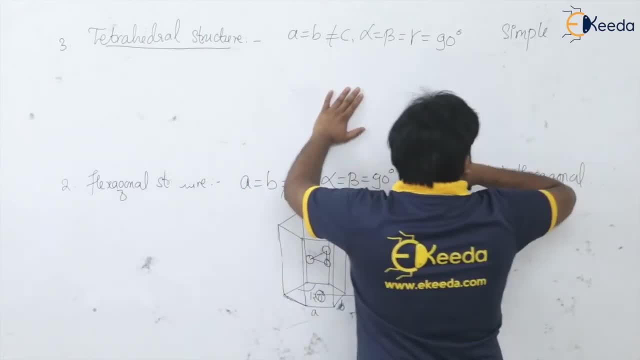 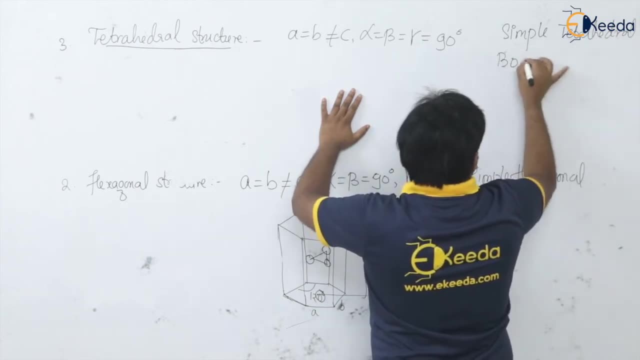 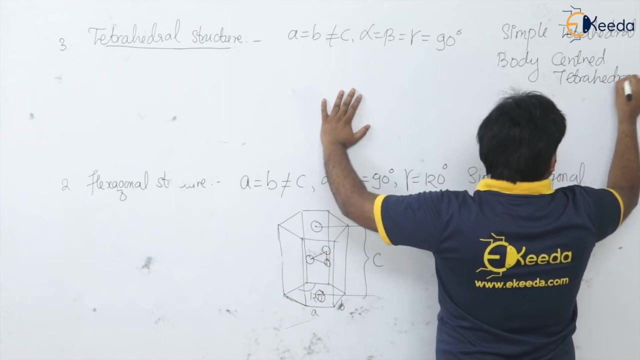 and the lattices we are having here, simple tetrahedral and body centered tetrahedral. tetrahedral, that is b, c, t, body centered tetrahedral, which is the crystal structure. So in tetrahedral structure, again same, this a is equal to b but not equal to c. 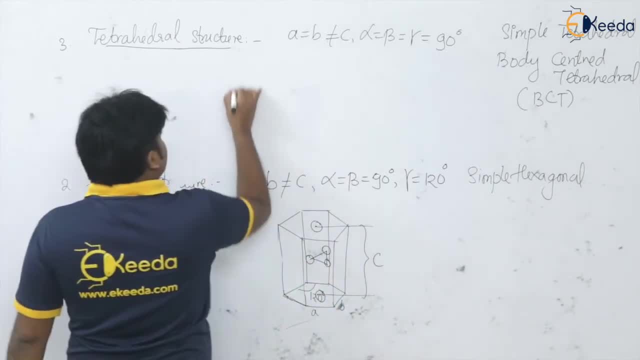 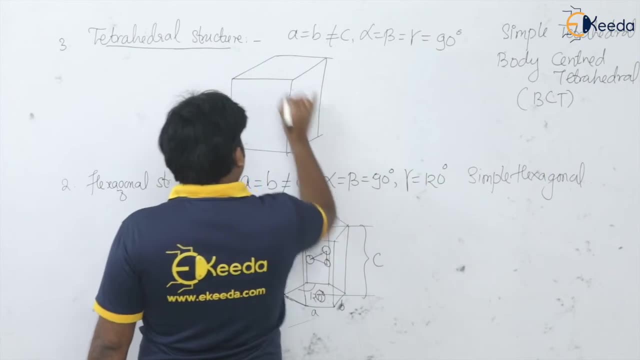 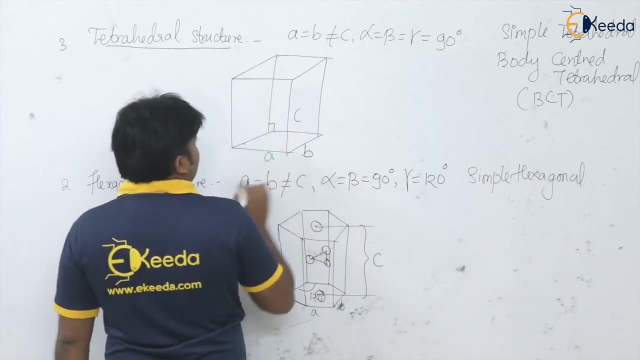 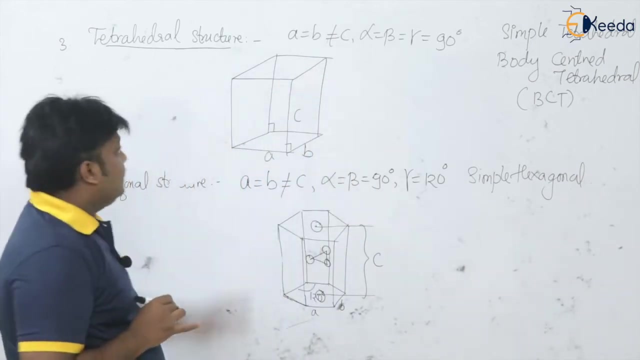 structure of the martensite. So here see, it will look like this: ok, this is a, this is b and this is c, and all the angles are 90 degrees right. So this is the body centered tetragonal. this is the b, c, t body center. sorry, this is the tetrahedral structure. 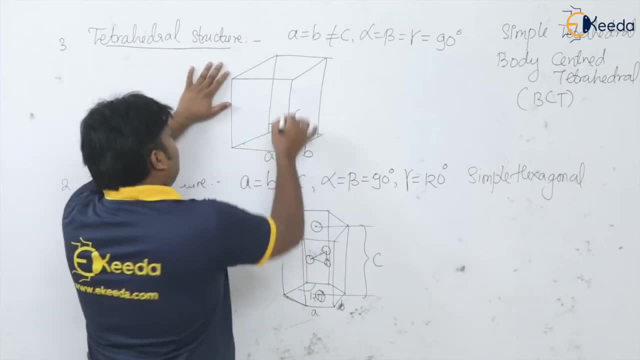 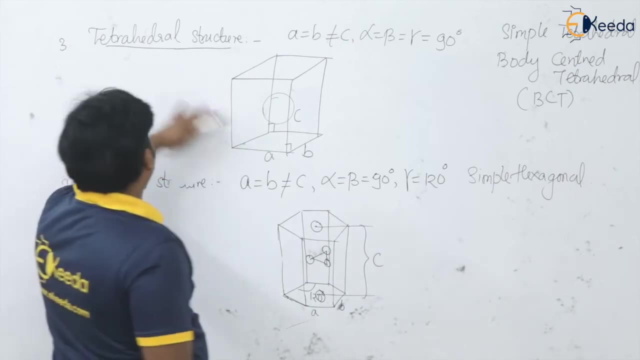 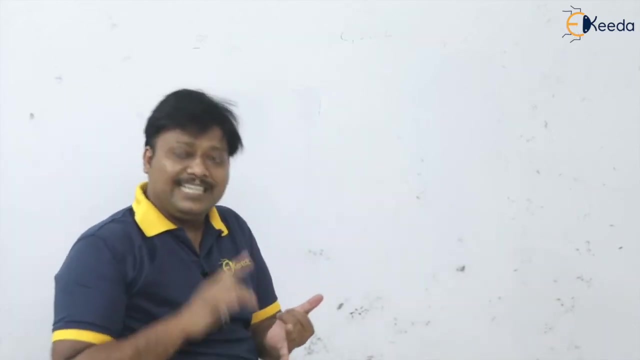 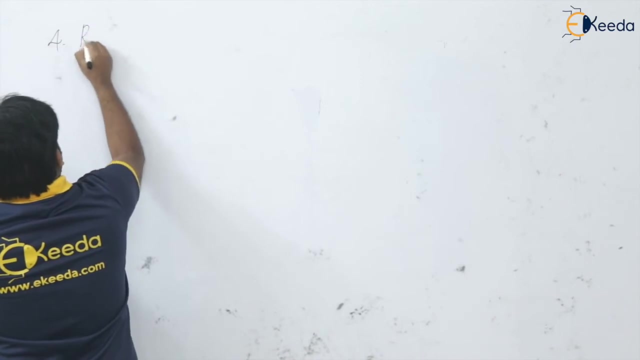 And this is the body centered, tetragonal. So body centered and at the corners. So this is the body centered, tetragonal, and which is the structure: tetrahedral structure. So we have seen the simple cubic, hexagonal tetrahedral. Now we will see the rhombohedral. this is our fourth rhombohedral rhombohedral. 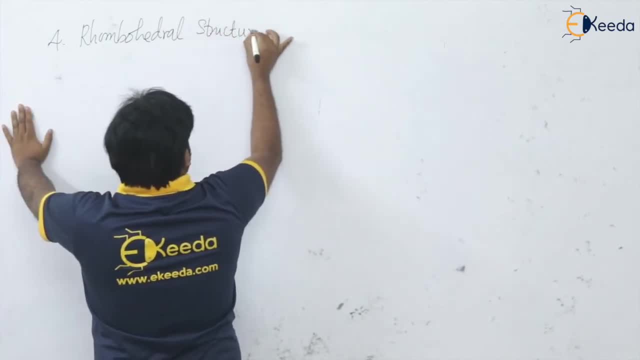 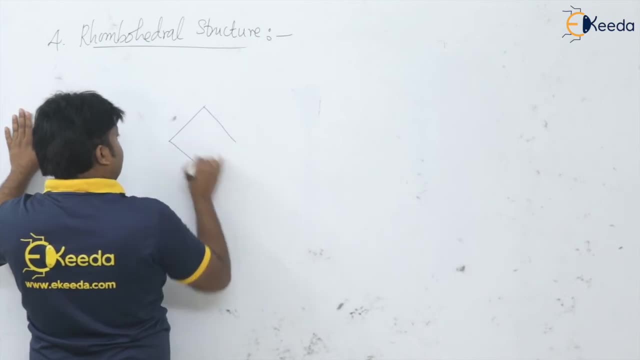 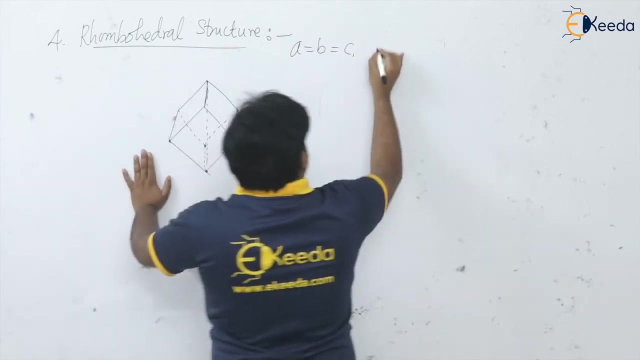 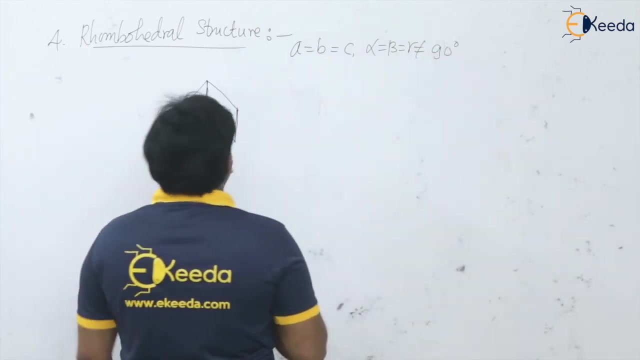 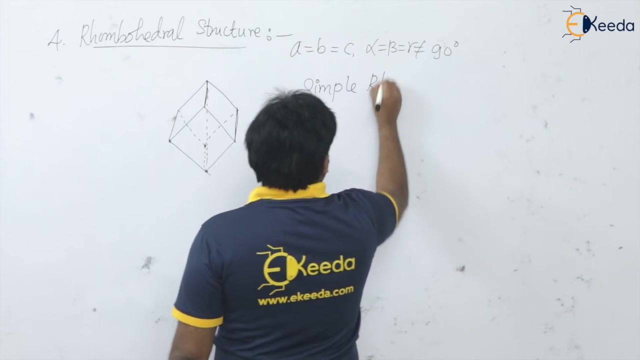 structure right. so how it will look like like this: so here a is equal to b is equal to c, but angles alpha, beta and gamma are not equal to 90 degrees. this is the rhomboid. and what are the lattices here? only simple rhomboid, simple rhomboid structure. 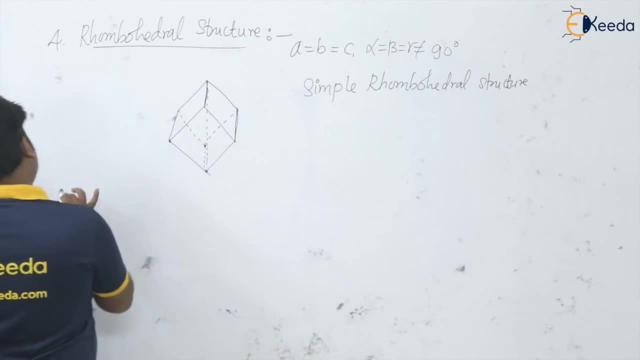 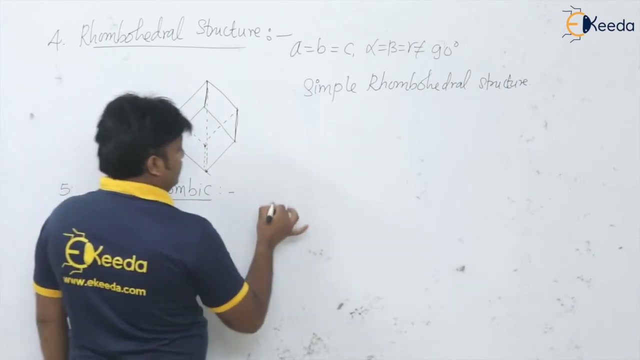 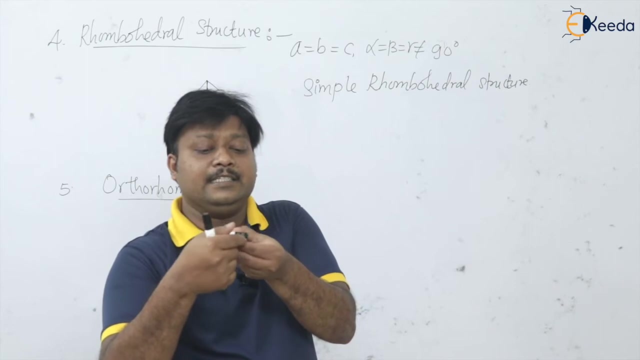 okay, so this is the rhomboid. then we are having fifties: orthorhombic, orthorhombic. so orthorhombic is like what? the matchbox. okay, so it will be like this here: say this is a, this is B and this height is C, like this ortho. 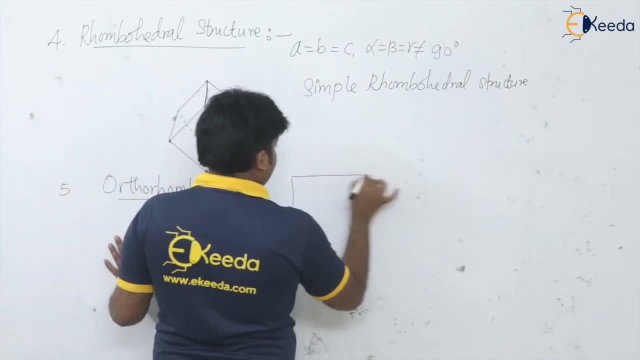 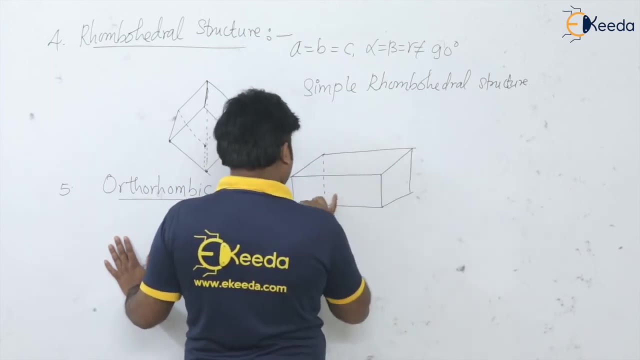 ortho, ortho, ortho, rhomboid, like a matchbox. so this is a, this is B and this is C. so here a is not equal to b, b is not, A is not equal to b, B is not equal to C, R is not equal to C, so that is it. but the 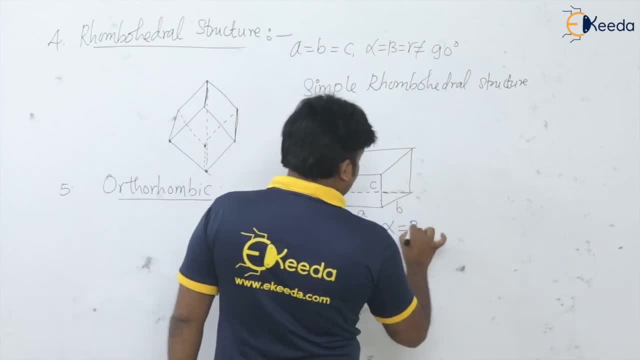 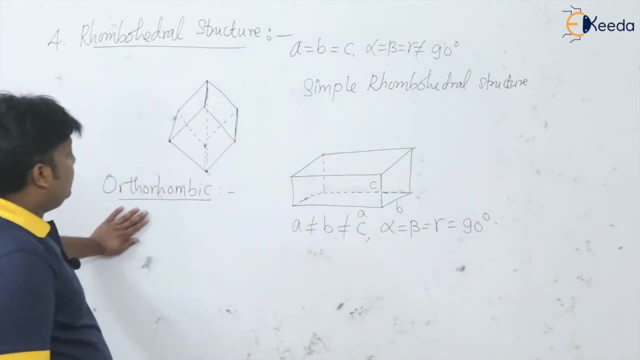 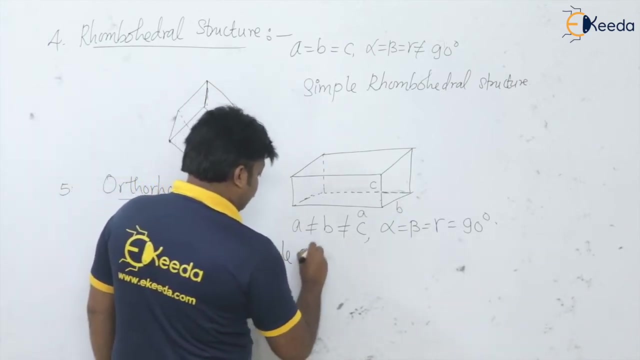 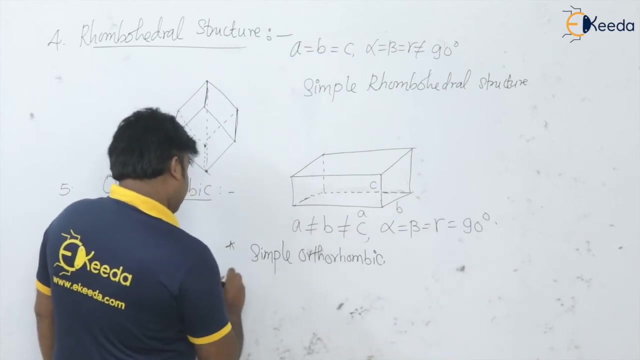 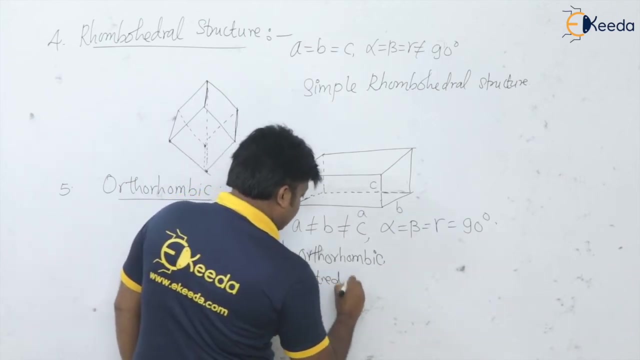 equal to c, but see the angles: alpha is equal to, beta is equal to, gamma are 90 degrees. and in orthorhombic crystal structure we are having what are the lattices? the simple orthorhombic, simple orthorhombic. then we are having the body centered, or thermic body centered, or four. 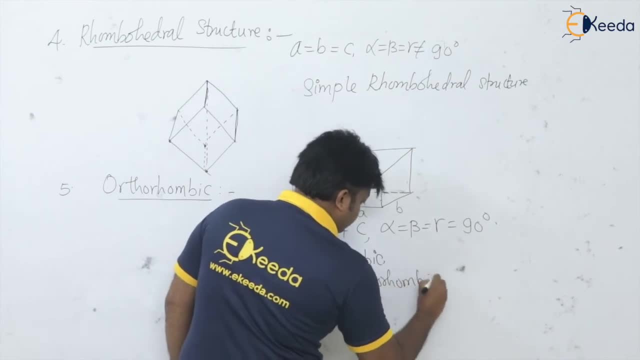 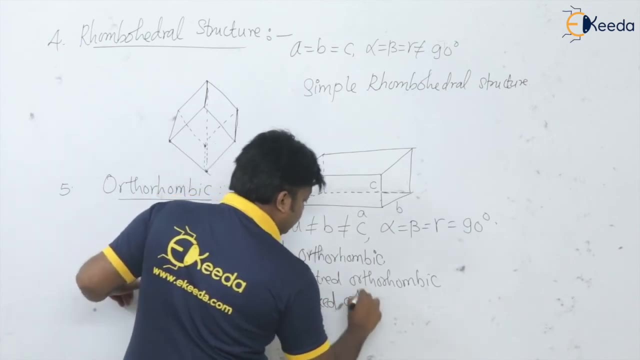 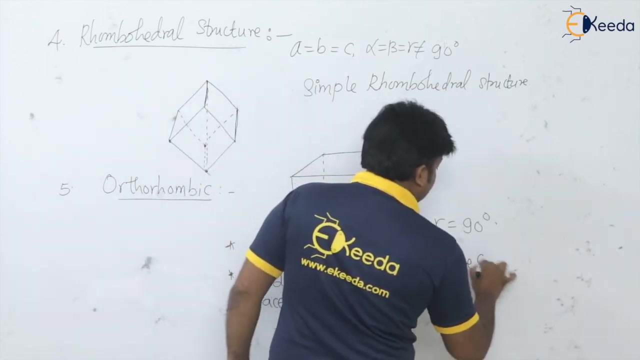 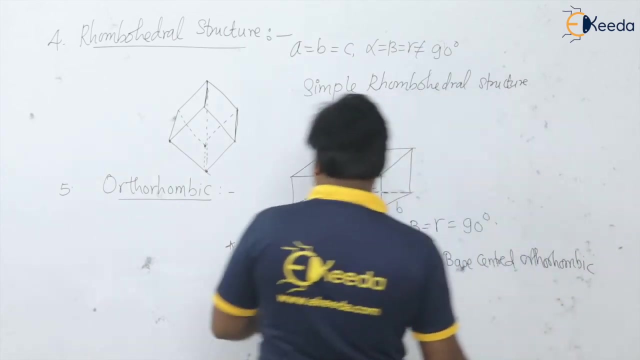 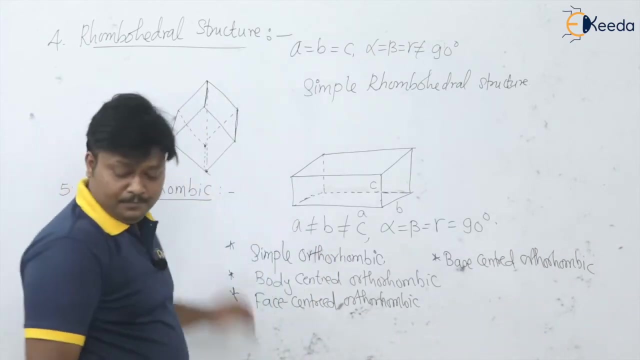 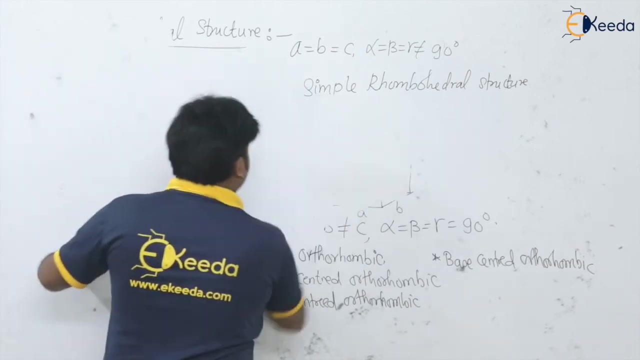 ombic, then we are having face centered or tour ombic and also we are having base centered, base centered orthorhombic. so in this we are having four lattices: one, two, three, four brevis lattices here. okay, so this is the orthorhombic. then the sixth crystal structure that we are 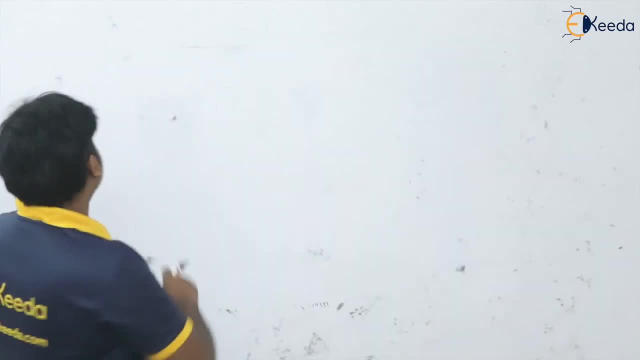 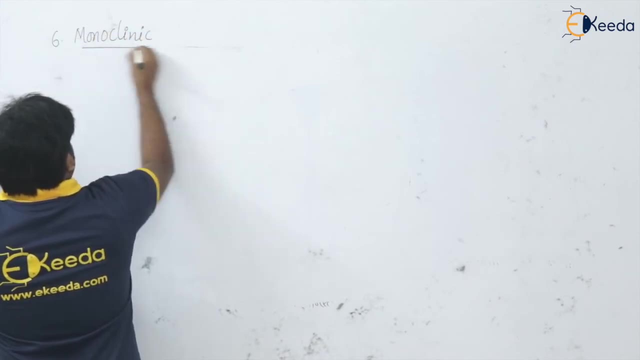 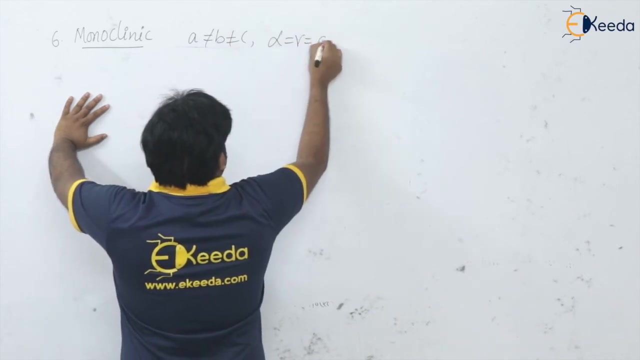 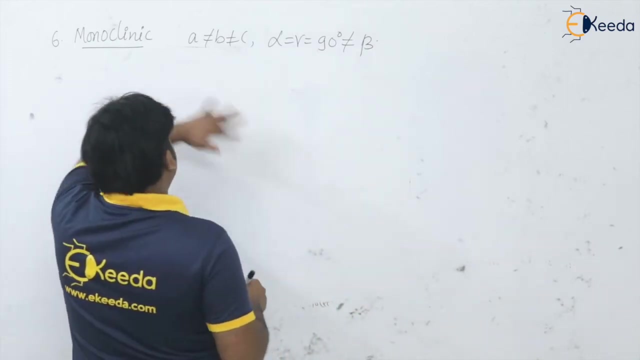 going to see is monoclinic, is monoclinic. I can see here: here: a is not equal to be, not equal. to see here: alpha is equal to gamma, is equal to 90 degree, but it is not equal to beta. this is a monoclinic structure. we can have this, a not equal. 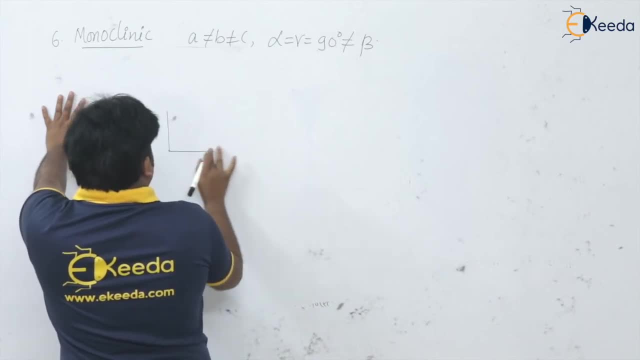 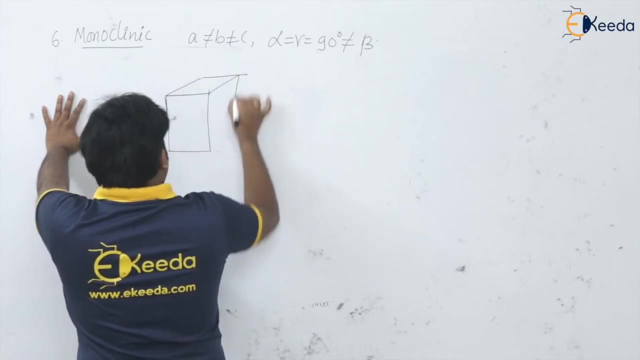 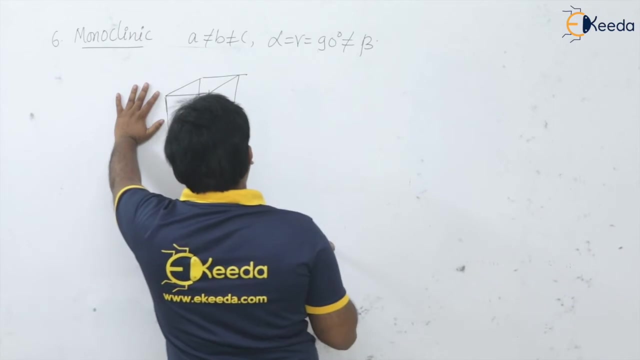 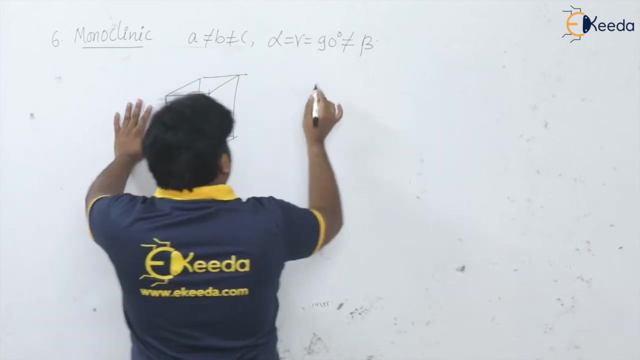 to b, a. so this is a, which is not equal to be, which is again not equal to C. so, like that, we are having the structure a, B and C and angles, alpha gamma are 90 degree but not equal to beta. this is the monoclinic structure, in that we are having the simple, monoclinic, simple. 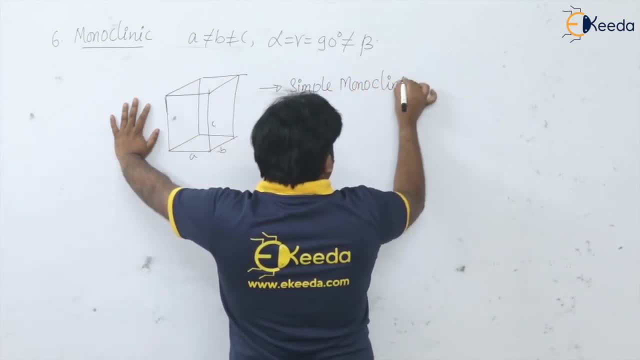 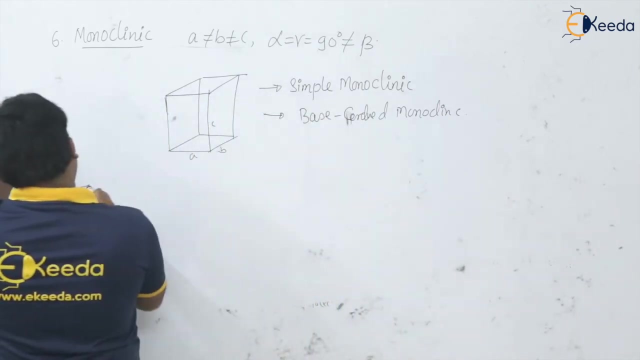 monoclinic and base centered monoclinic, bleep base centered monoclinic. right and last, this is the triclinic structure. triclinic, which is very difficult actually, because we need all these six like this, and we need all these six like this, and we need all these six. 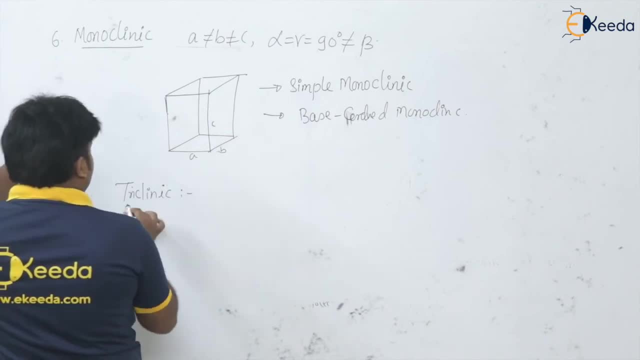 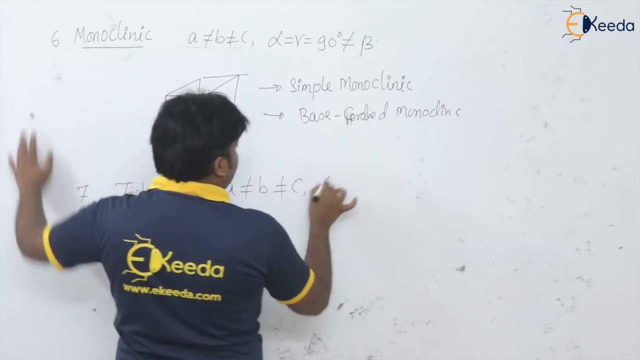 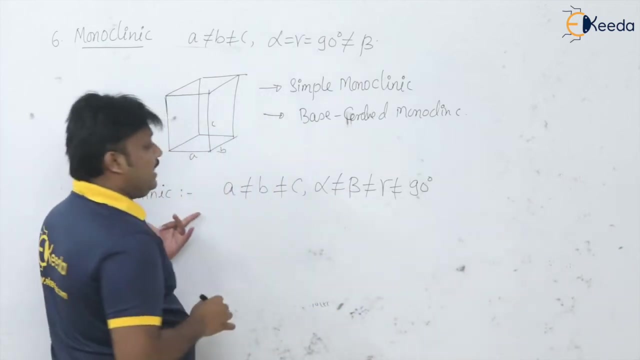 that is, parameters, ABC, and also alpha, beta and gamma. all are different. okay, here, a is not equal to B, is not equal to C, and even alpha is not equal to beta, is not equal to gamma, and they are not 90 degrees. so this is the triclinic crystal. 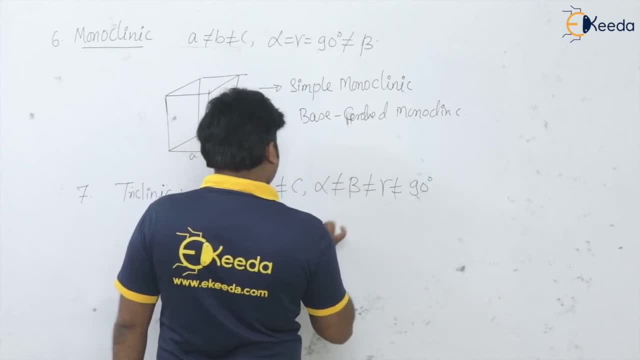 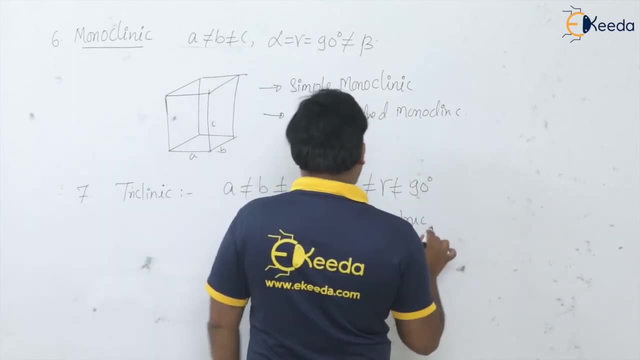 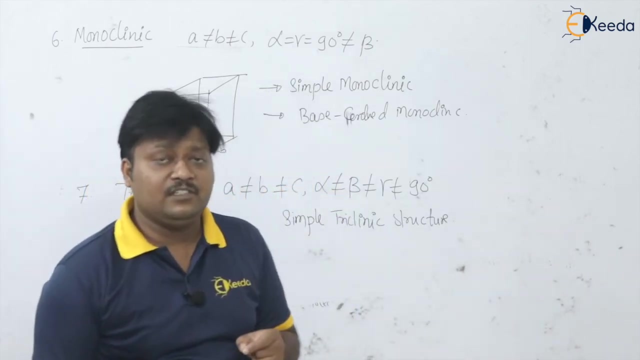 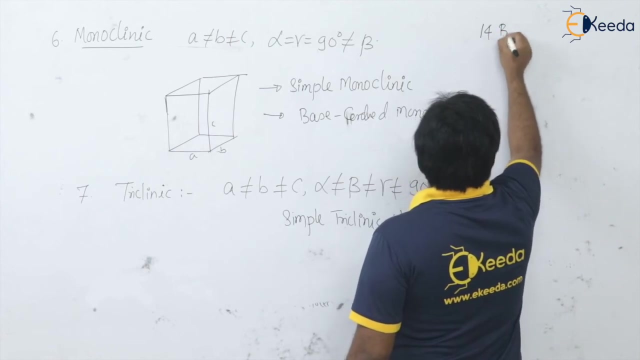 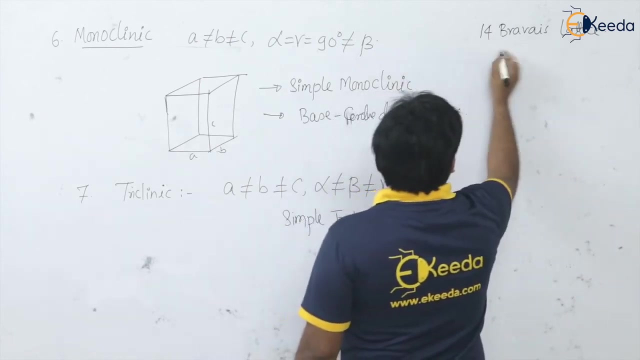 structure and in that we are having simple triclinic structure. okay, so like this we are having this seven. like this we are having these seven crystal structures, and if you count the fourteen braves, lattice, fourteen braves, lattice, con con sea thể in cubic, simple cubic. i will write in short then. 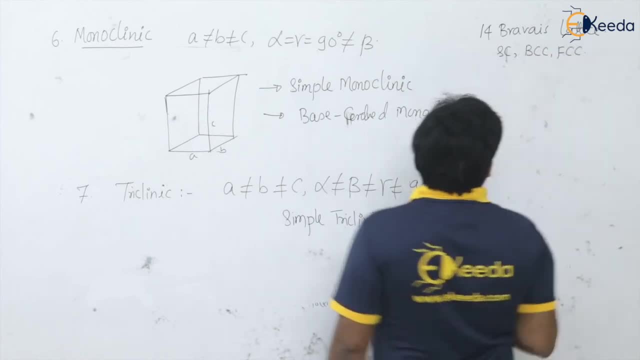 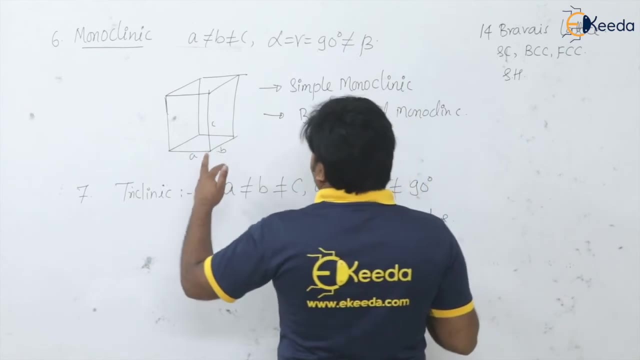 body centered cubic, then face centered cubic, isn't it in hexagonal matrix? and then 다른 curso, isn't it in hexagonal? we were having the simple hexagonal, then the tetragonal. we are having simple tetra tetrahedral, simple tetragonal actually, then body centered tetragonal, then. 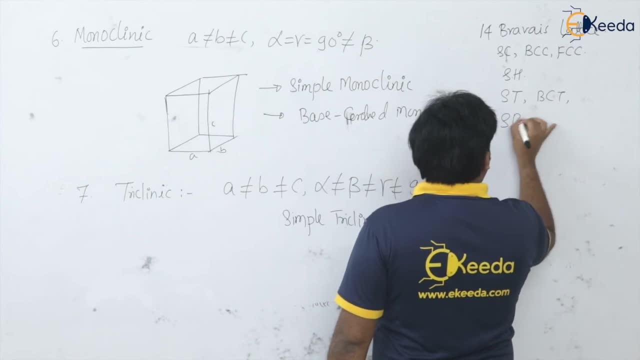 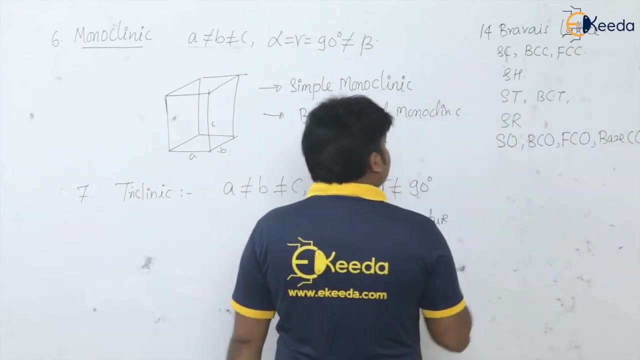 in rhomboidral we are having simple rhomboidral, isn't it then? we seen this orthorhombic there we were having the simple orthorhombic: body centered orthorhombic, face centered orthorhombic and base centered orthorhombic, isn't it then? in monoclinic, we are having simple monoclinic. 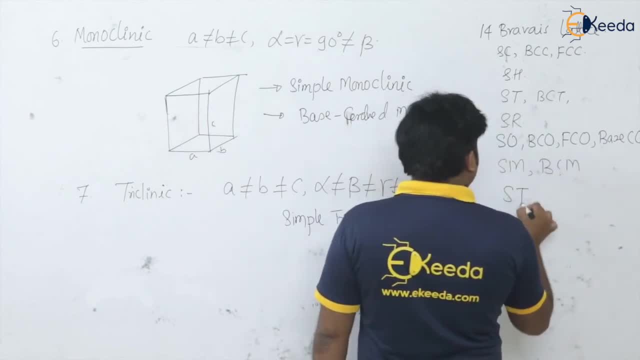 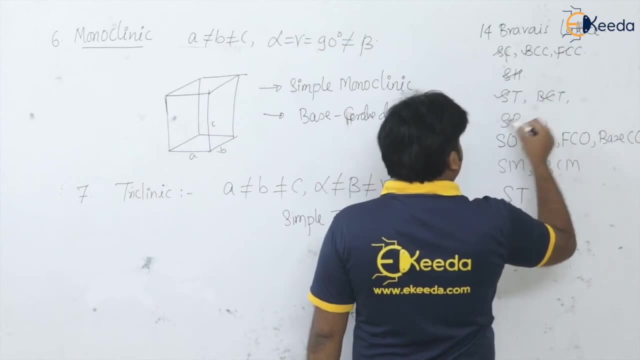 and base centered monoclinic and triclinic. we are having simple triclinic. so total 1, 2, 3, 4, 5, 6, 7, 8, 9, 10, 11, 12, 13 and 14. so these are the 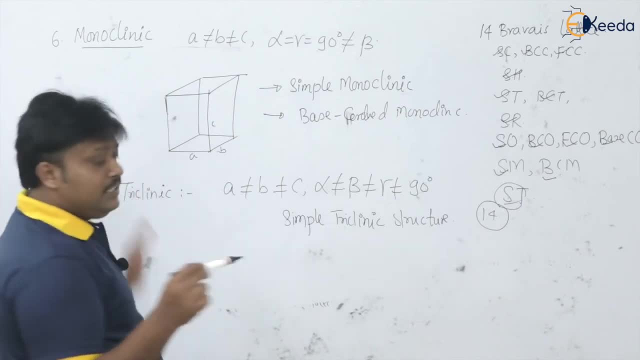 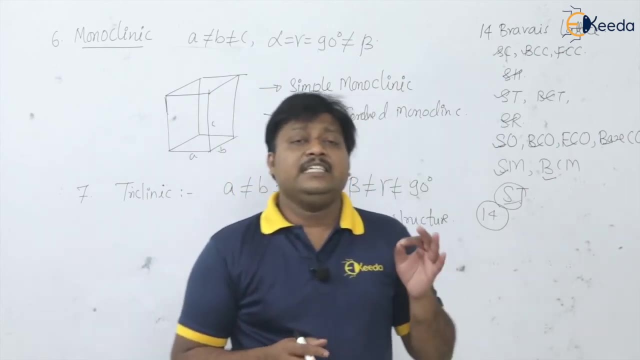 14 base arrays, arrangements or lattices for the 7 crystal structure. but see, dear students, most of the metals are having the cubic structure and for that reason we are going to see in details about the cubic structures. these are the simple cubic structure: face centered cubic. 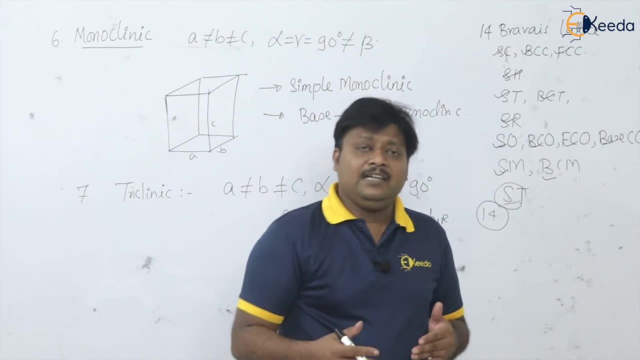 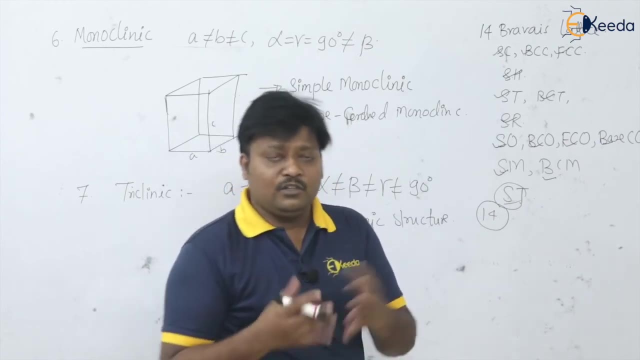 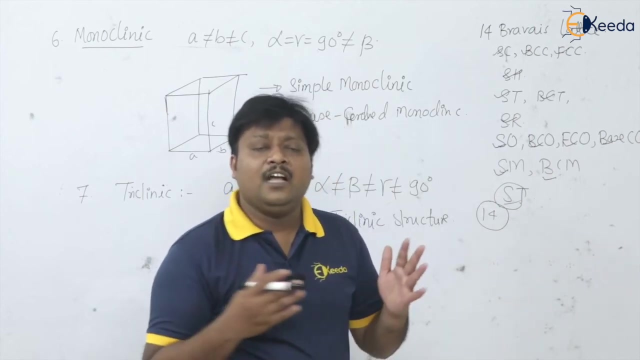 structure and body centered cubic structure and along with that we are going to see the hexagonal close pack structure. So for that we are going to find out the atomic packing factor, coordination number right, relation between the radius of the atom and side of the lattice, like that, these things. 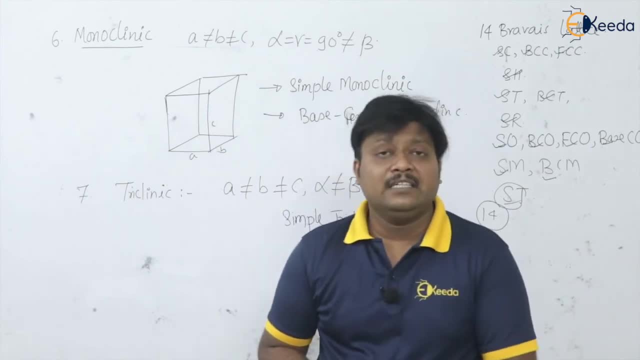 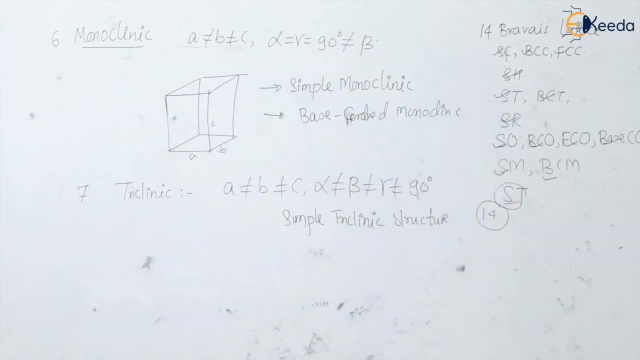 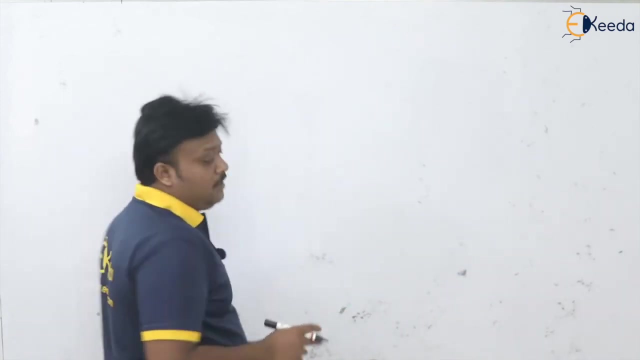 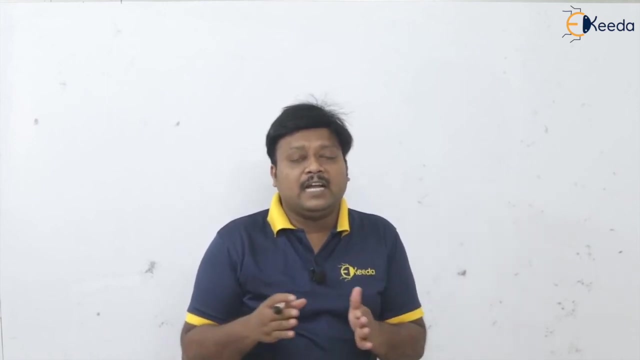 we are going to see basically for the cubic crystal structure. ok, so thank you, dear students. let us see the examples Of the various crystal structures that we have discussed for the cubic. so in the cubic we are having simple cubic, face centered cubic, body centered cubic, and also we are going 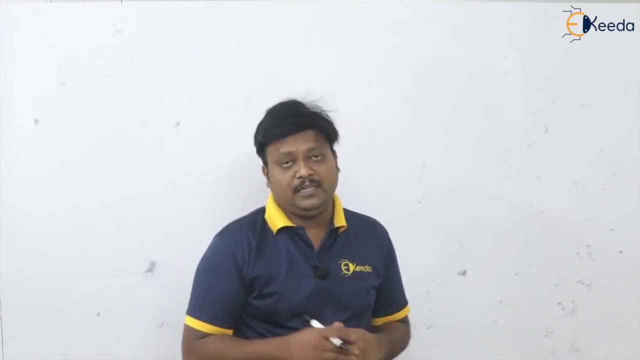 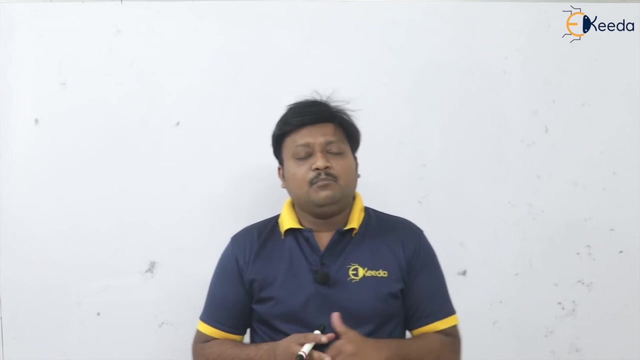 to see the examples for the hexagonal close pack structure that is HCP. So if you talk about the simple cubic structure, so there are very few elements of materials which shows that structure. the one of the examples of that that is the isotopes of the. 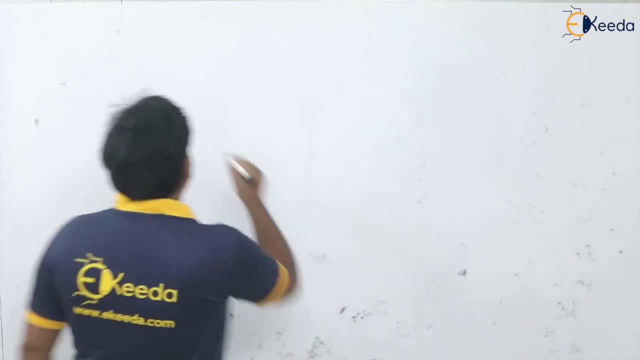 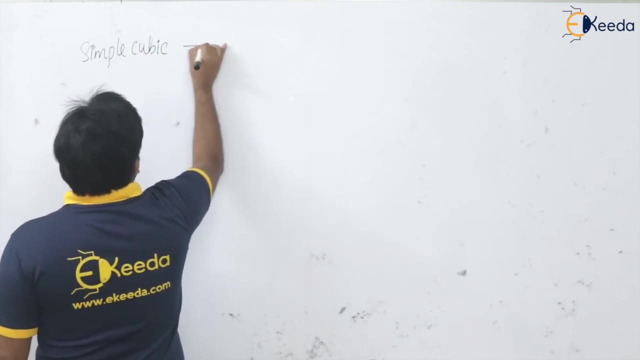 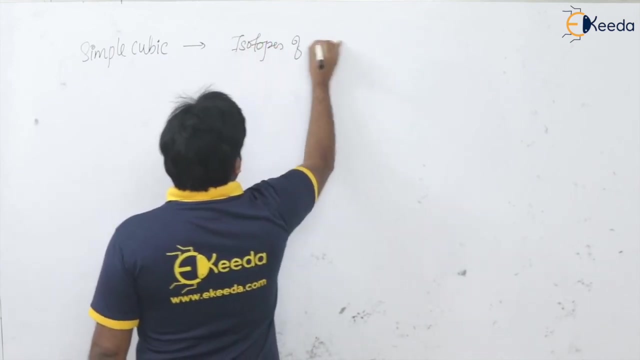 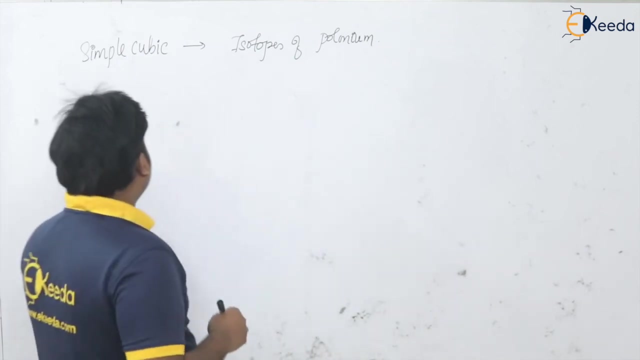 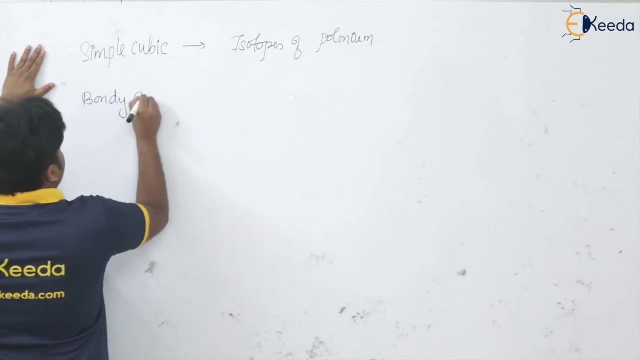 polonium, if we talk about the simple cubic structure. So what is the example for that? the isotope, the isotopes of polonium. This is the example for a simple cubic structure. Ok, the simple cubic. now, if I take the body centered cubic first, body centered cubic. 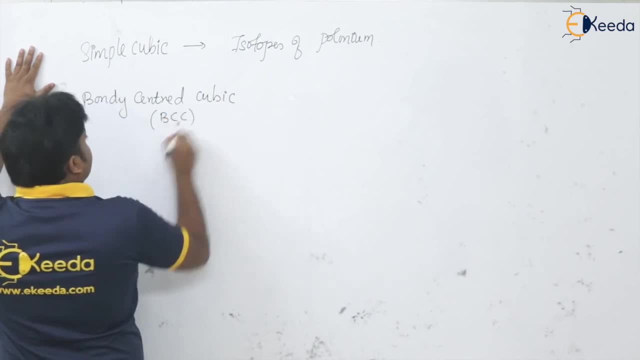 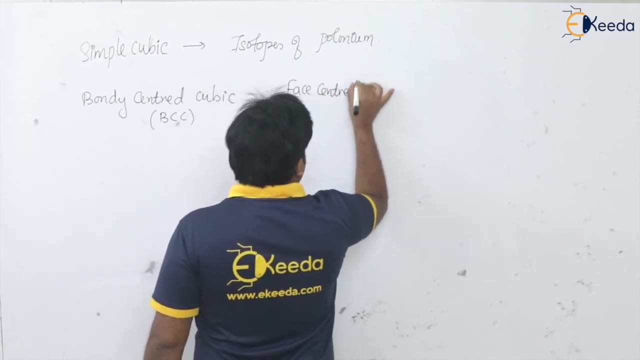 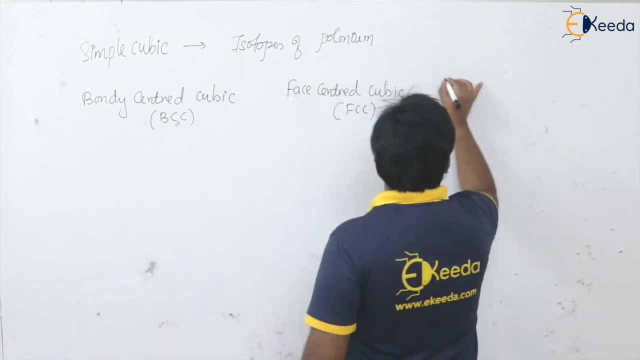 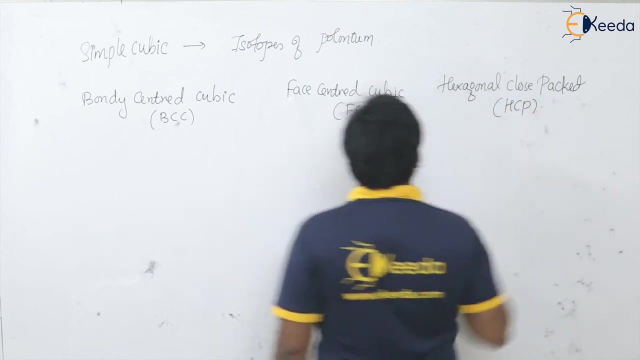 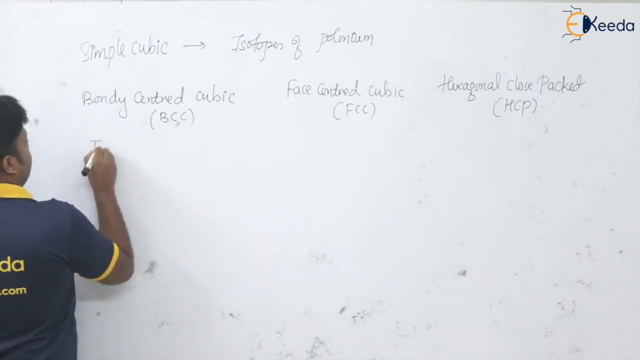 here I am having BCC. then I will take here the face centered cubic, that is FCC, and here I'll take the hexagonal clothes part structure, that is HCP. so in BCC we are having tungsten, chromium, vanadium, then sodium, we are also having the molybdenum and, if you see, the iron. 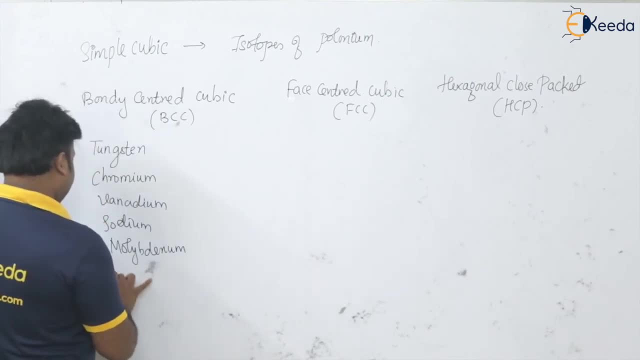 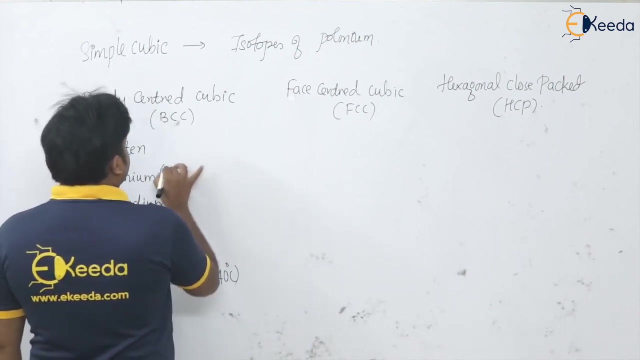 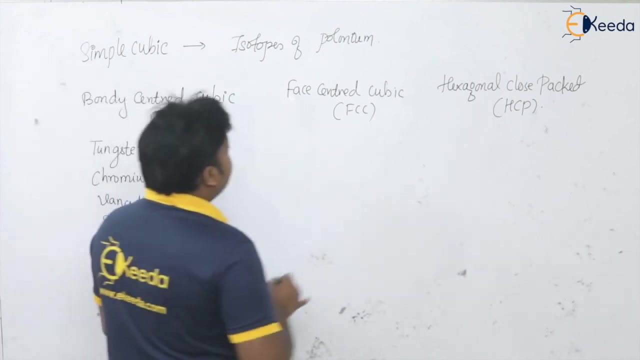 except in the range, except in the range of 910 degree centigrade to 1440 degree centigrade. that is alpha iron. you can say, okay, so these are some examples of the body centered cubic structures and which are very hard, very hard, isn't it? they are very hard if you talk about the face centered. 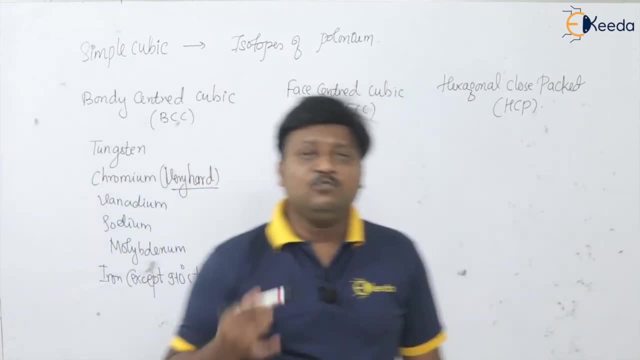 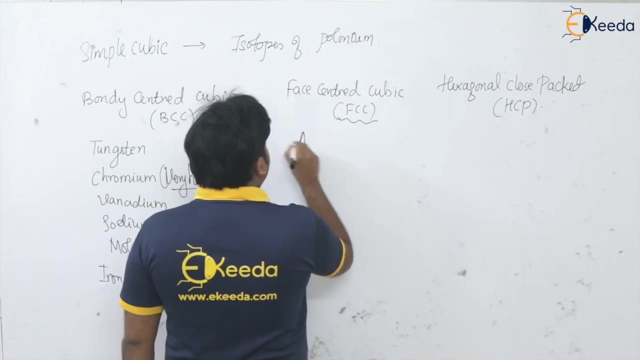 cubic structure, having good ductility, having good formability, that is epsilon. covalent imitability, that is FCC. Si Kone kohm, hi is May. we are having aluminum- here I mean copper- then we are having lead, we are having gold, silver, platinum and- very important- the gamma of P c would be кр. 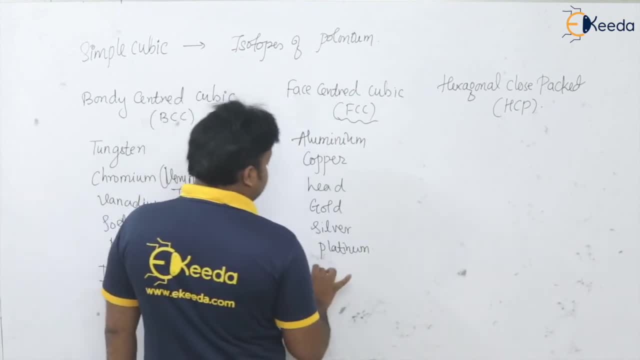 and very important. the gamma of P c would be: c would be fl. and very important- the gamma of P c would be: c would be fl. austenite. that is iron, isn't it in the range of 910 to 1440 degree centigrade? that is gamma austenite. 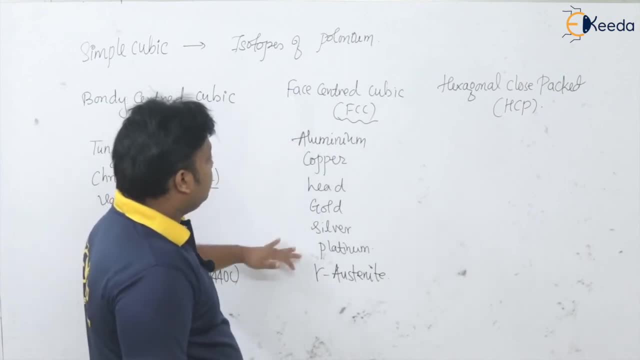 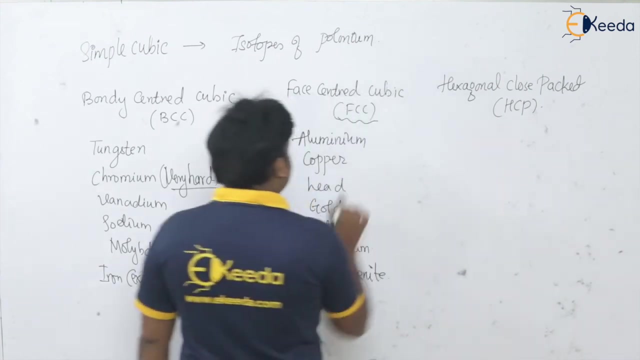 so these are the examples of the metals which are showing the face centered cubic structure. okay, so yeah, bcc, then fcc. we discussed for simple cubic and the hcp before that. these are what more ductile materials. please remember these are more ductile. then you talk about the hcp. these are zinc. 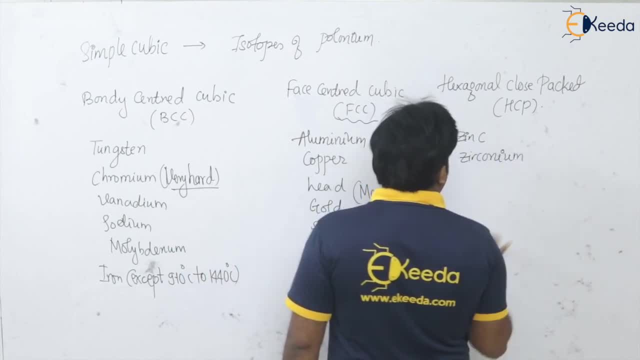 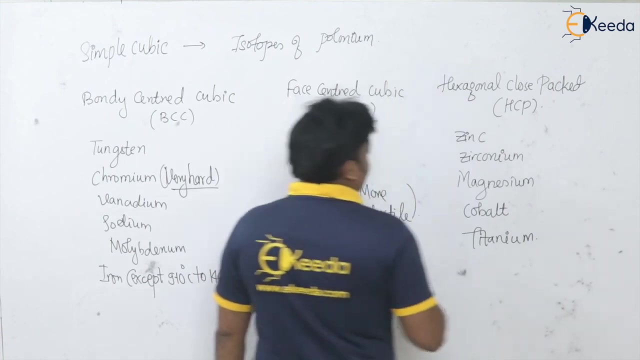 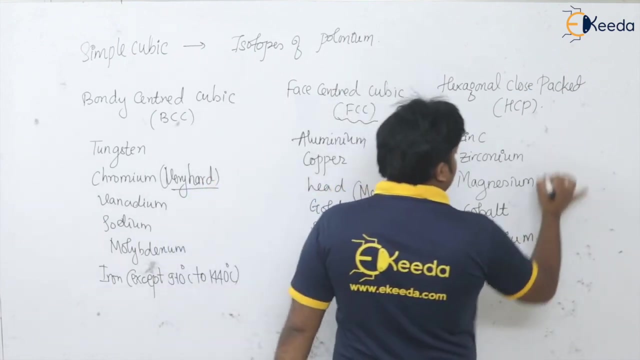 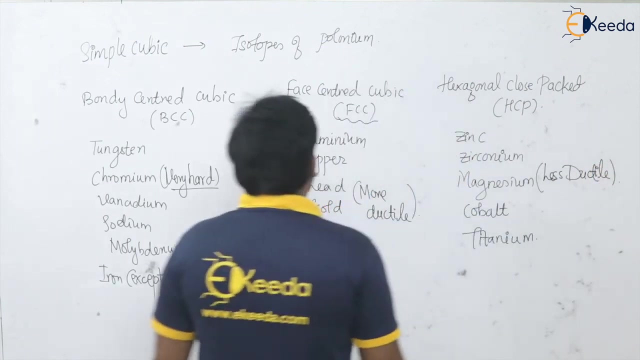 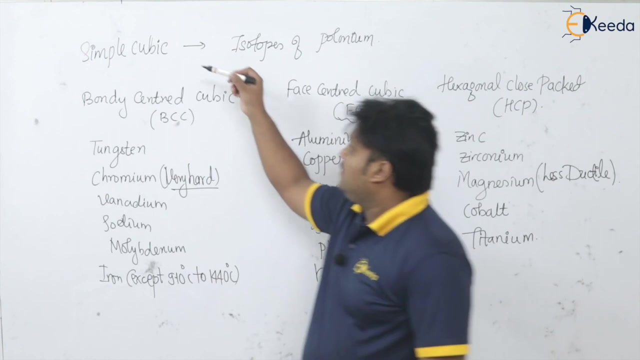 zirconium. then we are having magnesium, cobalt, titanium. okay, so these are the examples of hcp structure, hexagonal pack structure, and these are very important: less ductile, less ductile. so in this way we can remember the crystal structures and their examples actually. so these are their examples. this is, these are bcc, fcc and hcp and very few. the isotope of polonium belongs to simple cubic structure. thank you, you, you, you, so you.